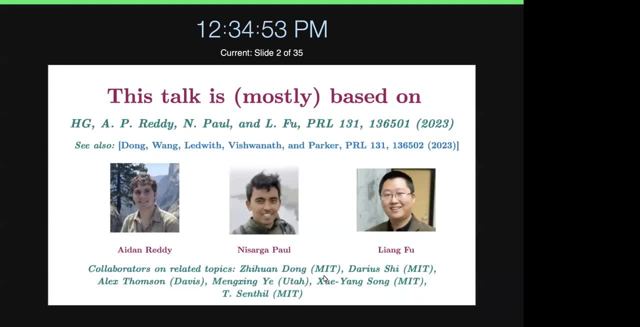 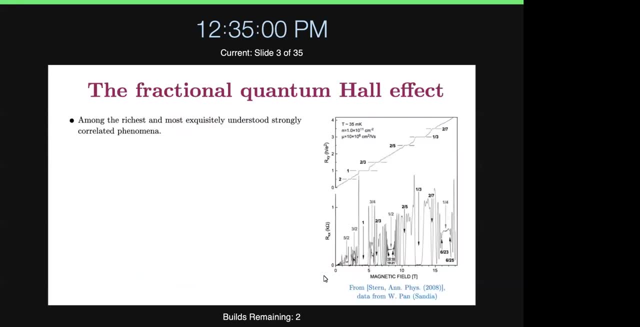 I also want to acknowledge several collaborators on issues that are related to the ones I will discuss in this talk. Yeah, is somebody trying to ask a question? No, okay, So I'll start with some general philosophical musings. I guess All of us know that the fractional Hall effect is one of the most rich and beautiful. 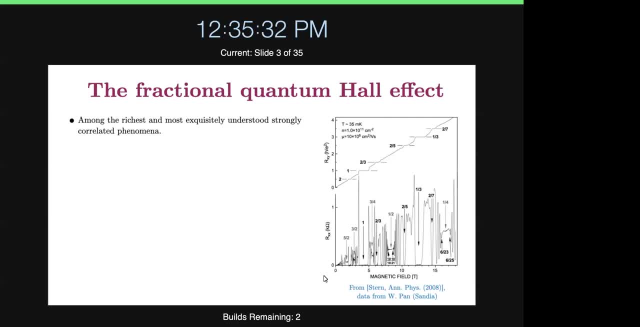 but also well understood strongly correlated phenomena in quantum matter. We understand actually a massive amount compared to a lot of other correlated systems in nature. In particular, we know ground state wave functions of quantum Hall phases. we know their universal responses, exotation spectrum and even we know 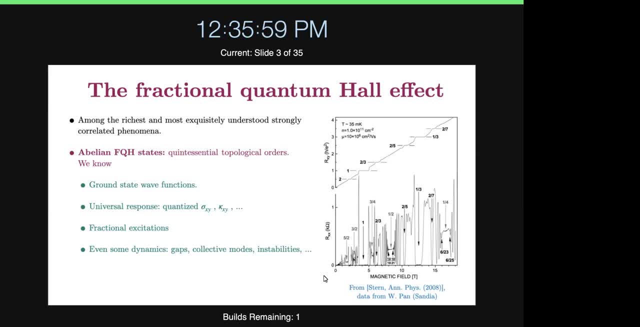 quite a lot about their dynamics, And even with this amazing understanding of quantum Hall, turns out that all of this beautiful physics is actually fairly hard to find, And one of the main goals of modern quantum condensed matter physics has been to try and find situations which are realistic, in which 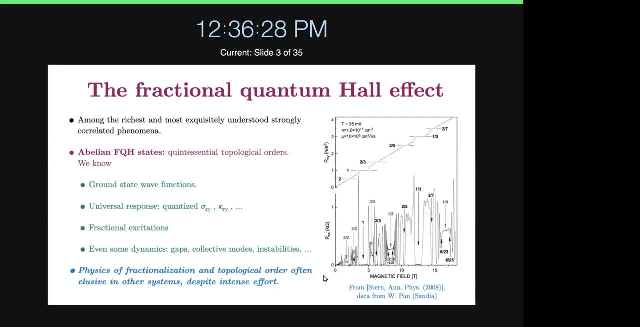 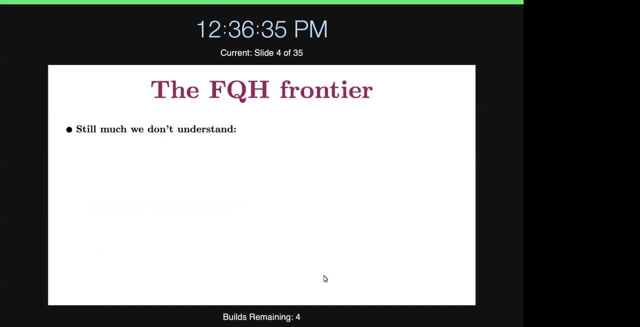 the physics of fractionalization and topological order can arise beyond the quantum Hall effect. So in spite of this, I want to emphasize that, okay, we don't understand a lot about quantum Hall, but there are actually many still deep and beautiful open problems just in the original. 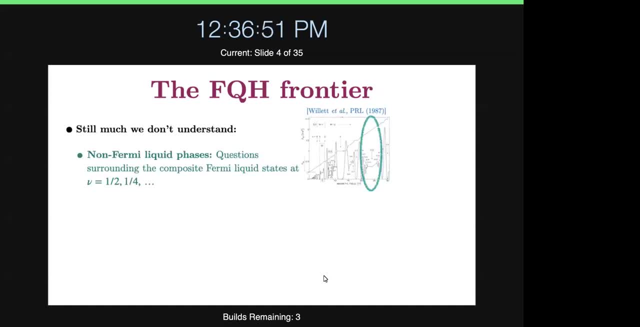 quantum Hall context. So in particular, quantum Hall is one of the poster children for realizing a non-fermi-liquid phase. So if you're filling one half, say in gallium arsenide, or filling one fourth, any even denominator filling, 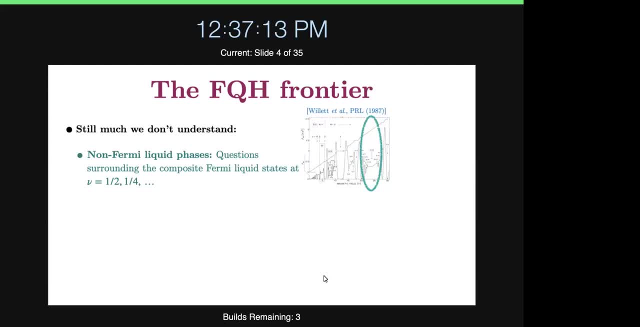 I will realize a metallic state. So you see the spinite conductivity feature here that I circled, because that's rho-X-X there, which we now understand in terms of composite fermions strongly coupled to emergent gauge fields in a manner that is that kills off a lot of the 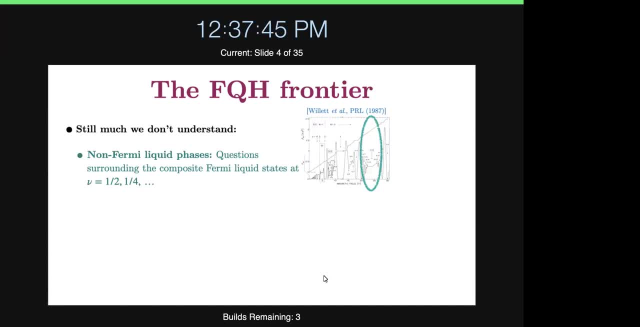 quasi-particle excitations. In terms of at least a theoretical understanding, this is probably one of the best understood non-fermi-liquids in nature, yet many of its grand state properties are still mysterious. There are also many things we don't understand about quantum phase transitions. 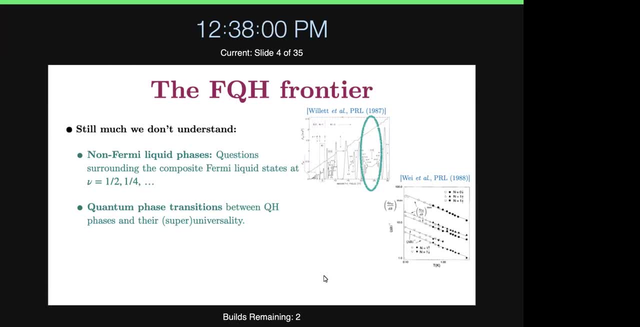 even in the traditional quantum Hall setting. So, in particular, if I think about transitions between different quantum Hall plateaus, experiments show that they actually all have and all happen to share the same critical exponents: new equals seven thirds andészz equals one. 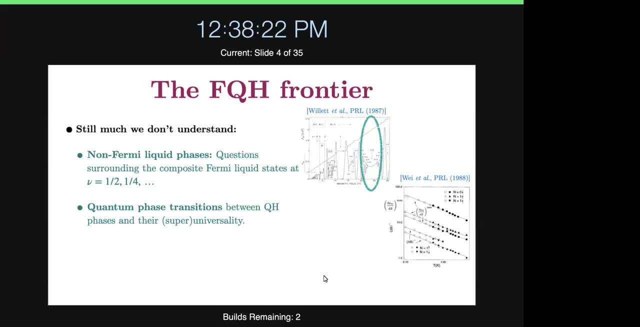 and at least in the integer transistors you can pantaglom the most fractional常 transistors is the product of n, MINO and z being consistent. That's well, we can't explain those exponents together with any systems. and secondly, 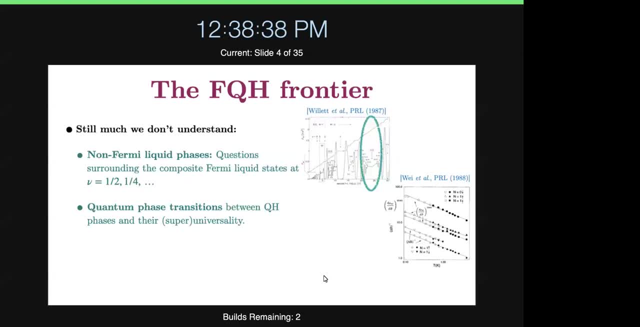 the fact that you have all of these quantum face transitions between totally different phases all sharing the same critical properties is a complete mystery that still has not been solved. Having gotten to their universal transport properties, that we've also not explained, they all have a universal 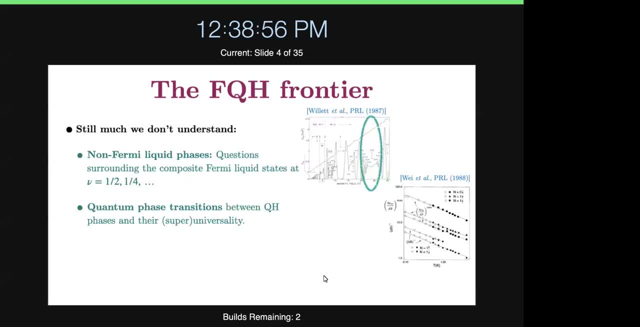 value of sigma xx and sigma xy, that no model has been explained, And also, I think, something that is near and dear to many of us is the question of how to generate interesting non-evolving states, And still, actually, there's a remarkable amount that we don't understand. 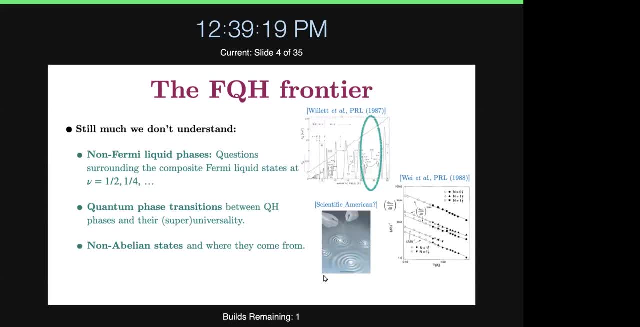 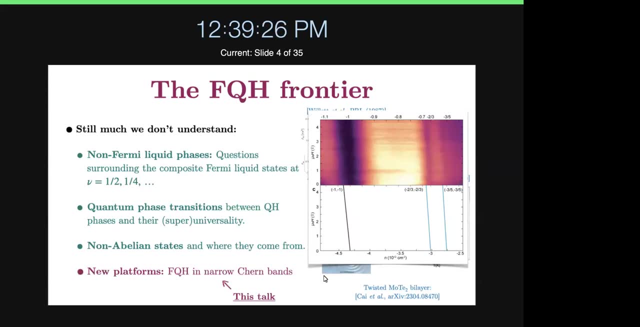 in this area, But the main focus of this talk, nevertheless, is going to be new platforms for exploring quantum physics. So I'm not necessarily going to solve these problems, but I'm going to talk about a new context in which, at the very least, we will learn more about them and also introduce 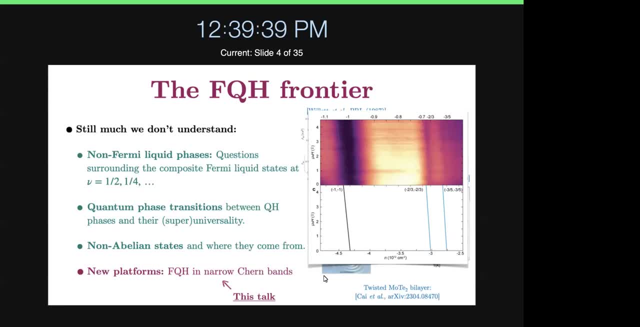 new problems, And this is the context in which we will learn more about the context in which we will learn more about the fractional quantum Hall effects in narrow turn band systems. So there was this amazing measurement which I drew up a plot from here on the right, 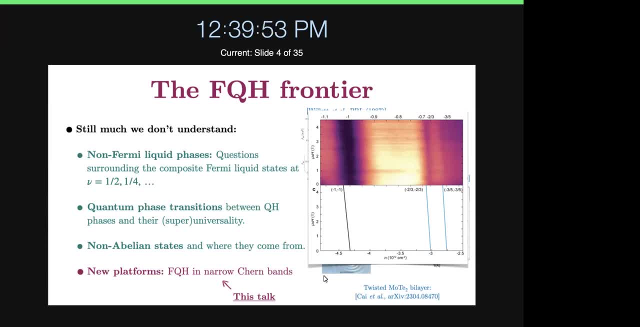 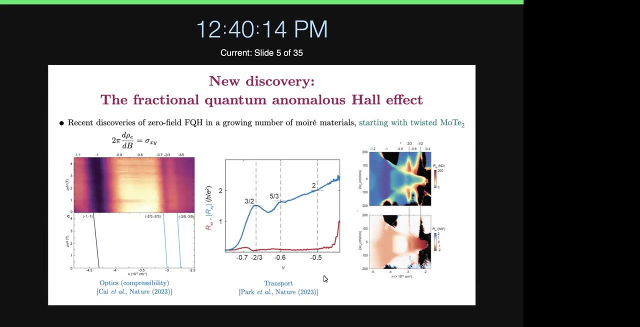 I guess several months ago, in April, demonstrating the existence of incompressible features at fractional billings of a narrow turn band in a twisted TMD system, This TMD system being moli ditaluride. So yeah, the special measurement which was a compressibility. 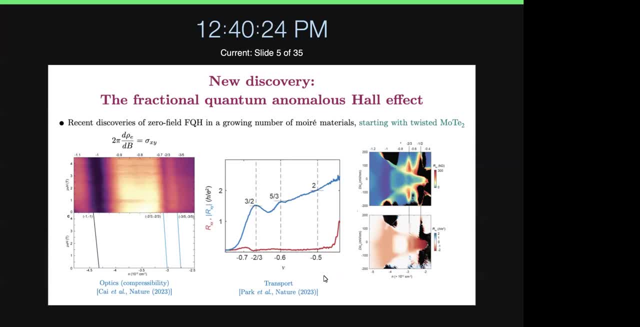 sees a minus two-thirds state, which we interpret via the formula here. So you can see these dark fringes here. Those are telling you that the compressibility is going to zero, And the slope of these curves which gives me d? rho by db here. 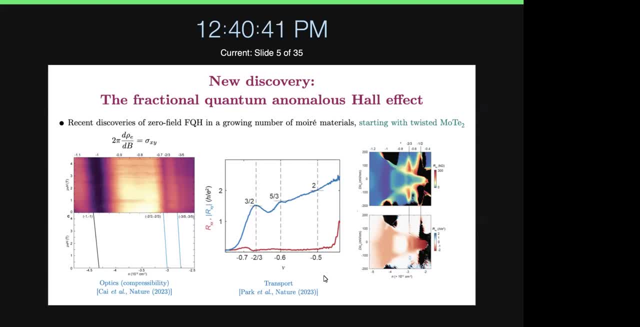 is going to be zero. So you can see here tells me the Hall conductivity. So you see a two-thirds state here and a three-fifths state. So I'm saying here, even though I'm actually not pointing on the zoom, but I'm pointing in real life. 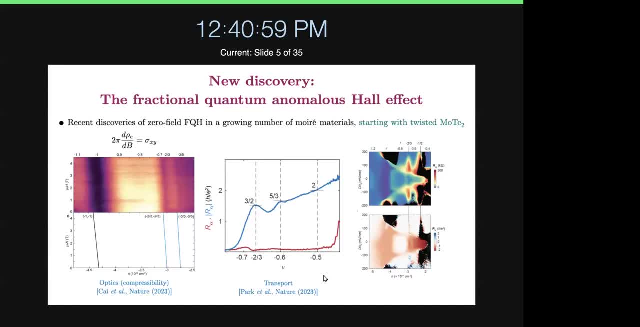 on the far right. So this was an amazing initial observation, And I think at the time we all thought: well, this is great, But of course, in order to confirm all of this physics, we still need something like transport. Now, amazingly, 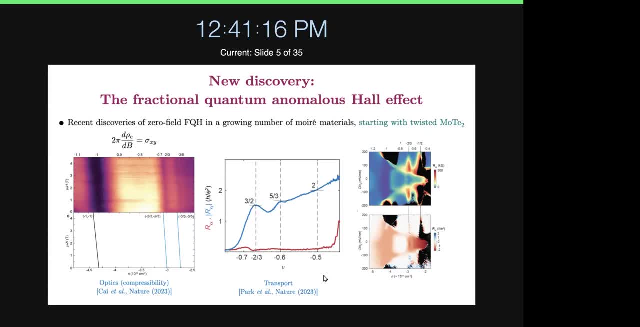 transport measurements did come out. They're shown on the right here from the same group at the University of Washington And you'd see features with reasonably good quantization of rho xy. The red curve at the bottom is rho xx. It doesn't show particularly amazing features here. 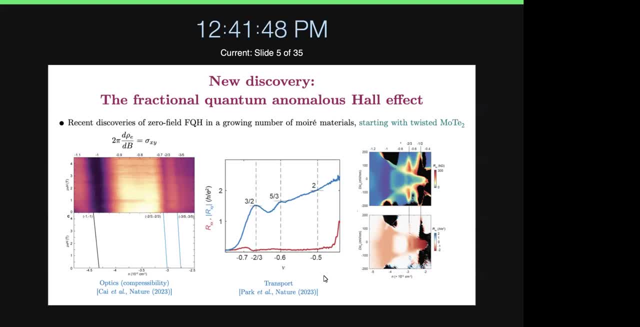 but rho xy. you see all kinds of interesting, at least somewhat quantized features at three-halves and five-thirds, Or sorry, two-thirds and three-fifths. This is rho xy. The filling is inverse of that And interestingly, 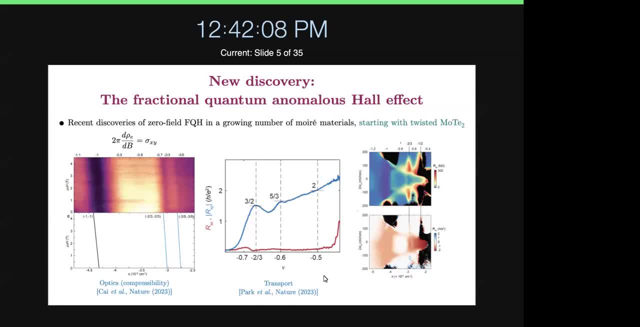 also observed is this feature where the whole conductivity or whole resistivity is close to two. All this, by the way, is in units of h over e squared, And the system seems rather metallic, which is reminiscent of this composite Fermi liquid that I was mentioning. 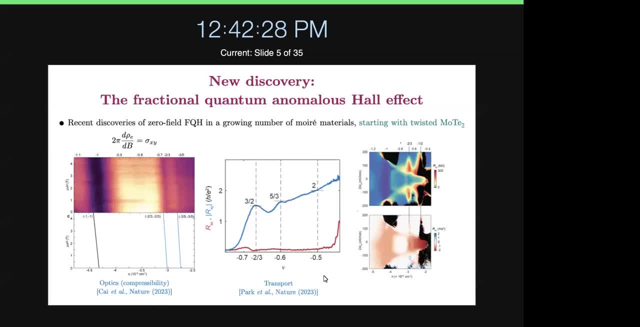 a couple of slides ago, And something that really is additionally amazing about this system is you get an additional tuning knob in the form of displacement field, which is an electric field perpendicular to the sample that essentially tunes the width of the flat churn band. that's realizing this physics. 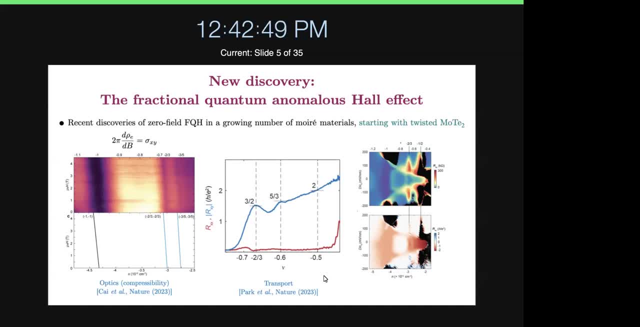 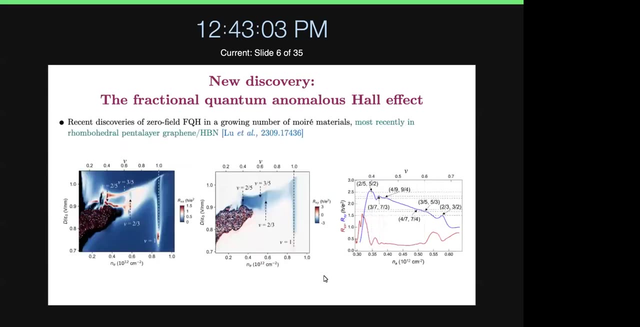 And you see transitions from quant-mall states to from these quant-mall type states to more resistive states, which I'll discuss in a bit more detail later. Okay, So even more surprising is, just recently, the same type of physics was observed in very 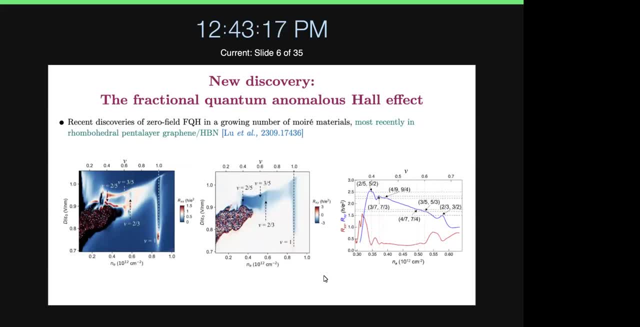 well, quite different material: rhombohedral pental layer graphene on HBN. So this is a graphene system rather different microscopics, And nevertheless they managed to find. this is from a group at MIT of Wang Ju, not just the two-thirds. 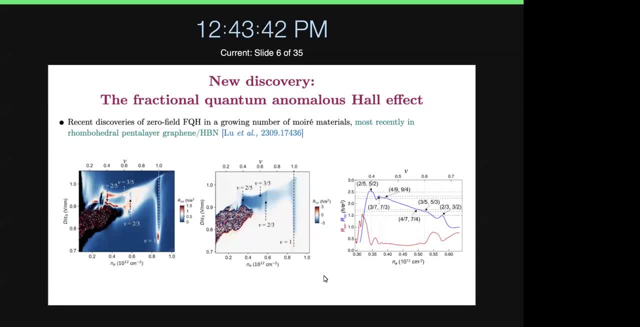 and three-fifths states, but also additional features which look like fractional quant-mall states in the hall resistivity at here it's three-sevenths and four-sevenths. So really really remarkable that in this system you see even more fractions. 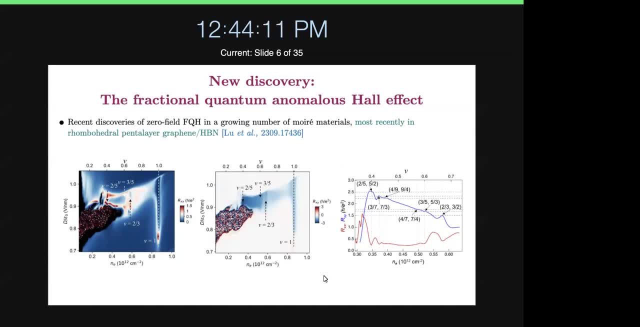 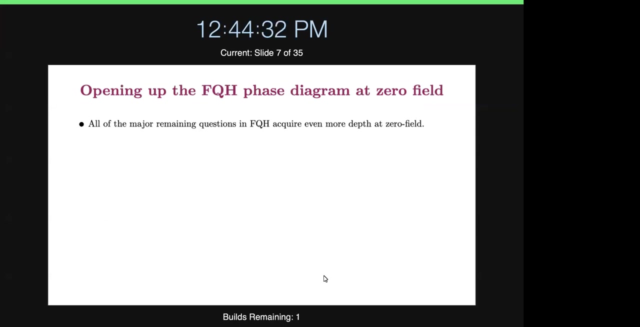 and also very similar overall structure to this resistivity plot to the TMT, which I always think is very surprising and is signaling that a lot of this physics is universal. Okay, So why be interested in this physics if it's just a quant-mall? 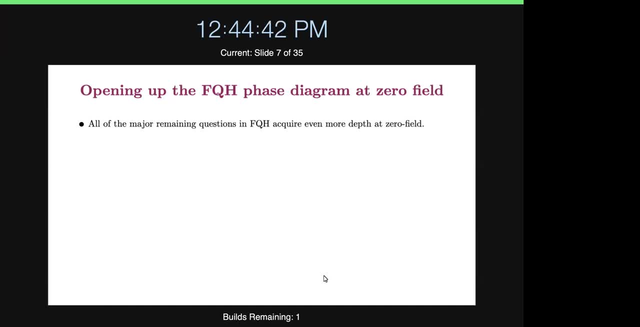 but it's zero field. Well, I argue that all of the big questions in quant-mall require much more character in the zero field setting. And the reason for that is: in ordinary quant-mall systems phase transitions are tuned either by filling or you imagine. 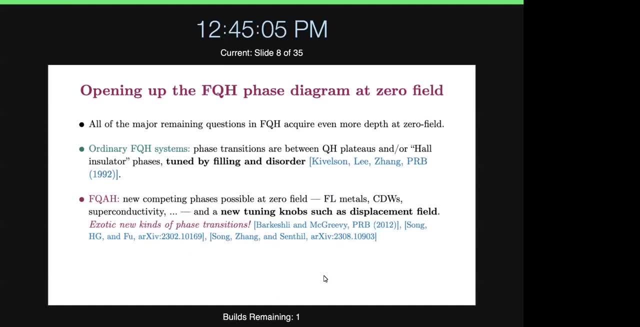 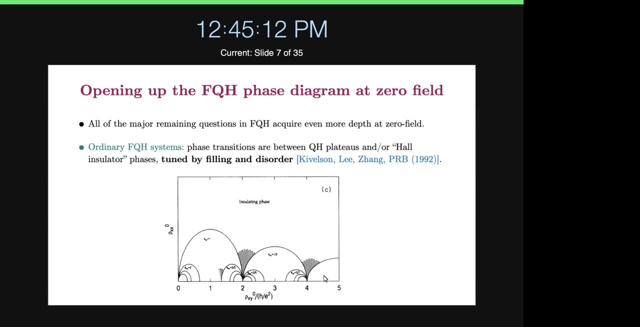 tuning them by disorder. So I can, you know access, go back here the sort of global phase diagram of the quant-mall effect with these two axes, you know rho-X-X here classically, I think, describing the. 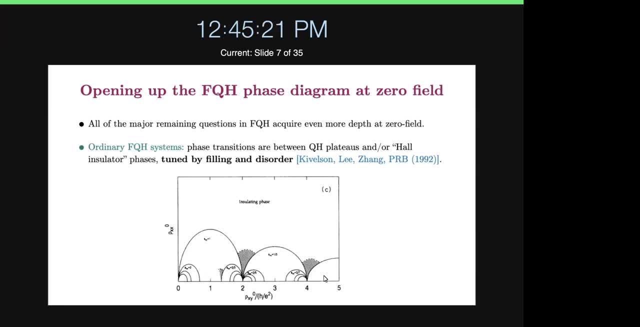 disorder and rho-X-Y you can think of as like a field direction here And we can then model different the landscape of quant-mall states using this overall picture, with these crosshatch regions, here being these composite Fermi liquid states, But in the zero field setting. 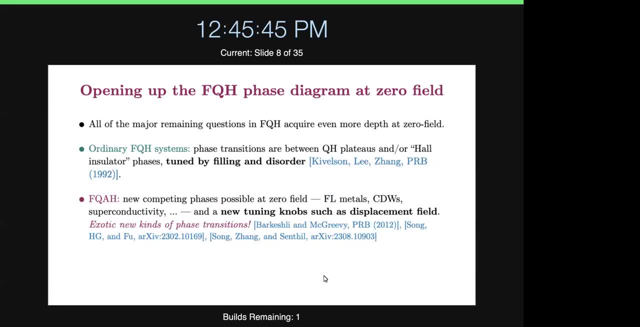 now we have this displacement field that I mentioned And we have all kinds of additional competing phases, such as Fermi, liquid metals and charge density waves and maybe even superconductivity that are also- which I already said probably two or three times- could lead to new exotic kinds. 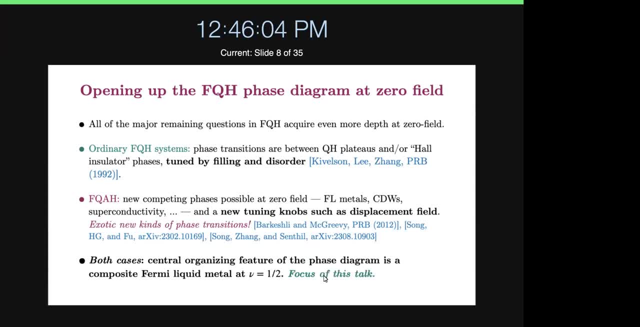 of phase transitions, And so I'm going to argue here with the rest of this talk, is that an organizing feature of the phase diagram in these systems is going to be a composite Fermi liquid metal. again, a nu equals a half, which I already 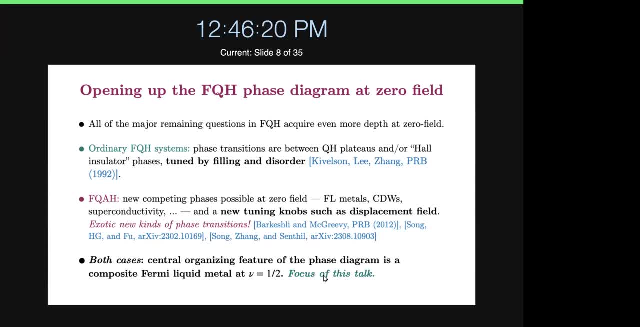 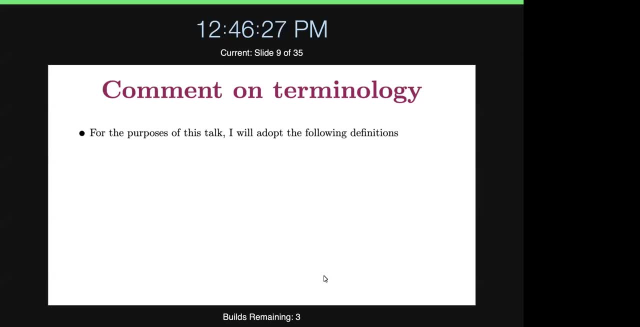 signaled to you guys in the earlier data. So before I get to that I need to acknowledge a certain question of terminology. So I've been saying fractional so far. I'm going to switch to using the phrase fractional anomalous to describe zero field states. 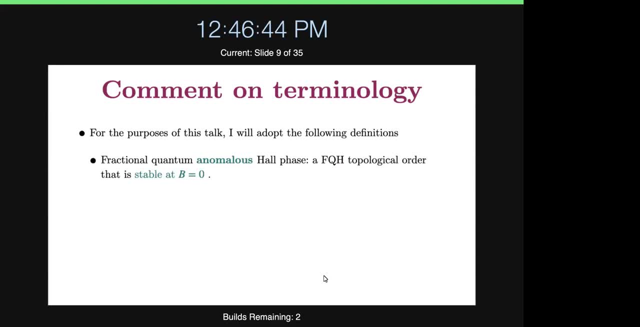 I happen to like that terminology as describing generally fractional topological order, which is stable in zero magnetics. Now there's an additional term which many people use as well in the setting, which is that a fractional translator. So from my point of view, 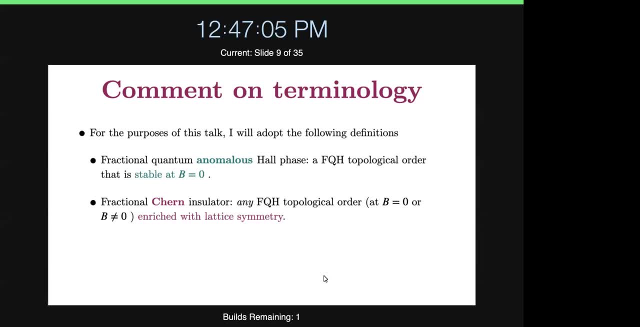 FCI is also a great piece of terminology that describes any fractional topological order, either at zero or a finite field which is enriched with symmetry of an underlying lattice. So we kind of need this as an umbrella term, at least from my point of view. 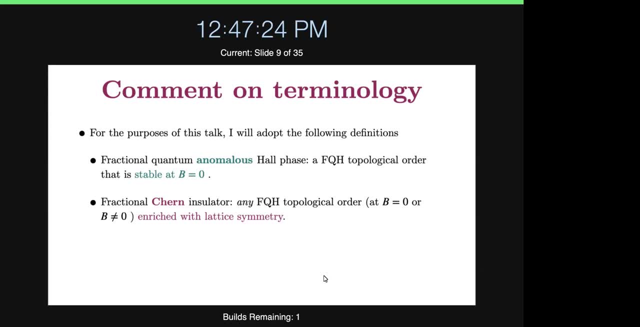 and FQAH describes something more specific, And so I'll maybe make the perhaps controversial statements that FQAH makes To me. all FQAH phases are FCI's, but it's not at least immediately obvious that all FCI's. 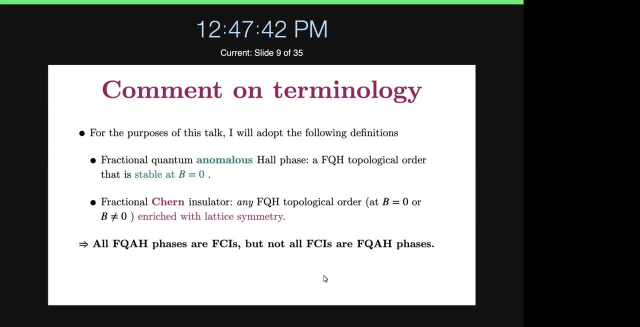 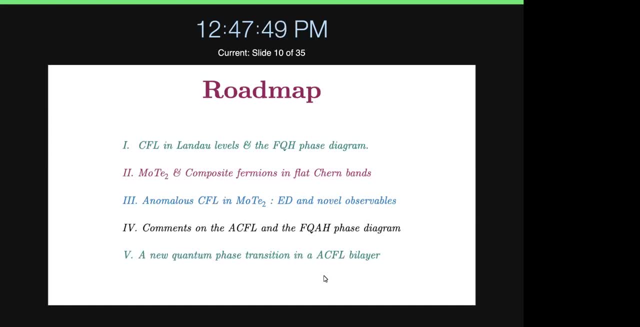 have a stable realization in zero field and in that sense are FQAH. Okay, So just a roadmap of the rest of the talk. First I will discuss the physics of the composite Fermi liquid in the Landau level setting and the use. 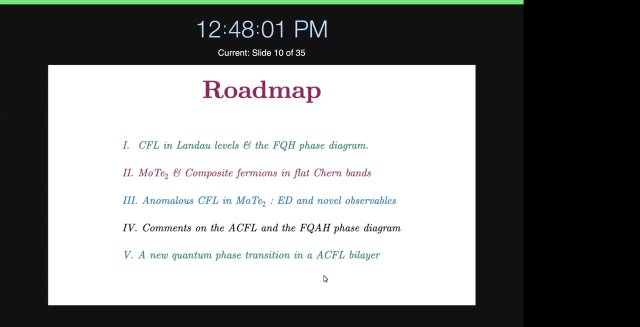 of composite Fermi on organizing the fractional Hall effect diagram. Then I will actually talk about the specific case of Mollet and Telluride and proceed to discuss the zero field composite Fermi liquid that can be realized in this setting, how it organizes. 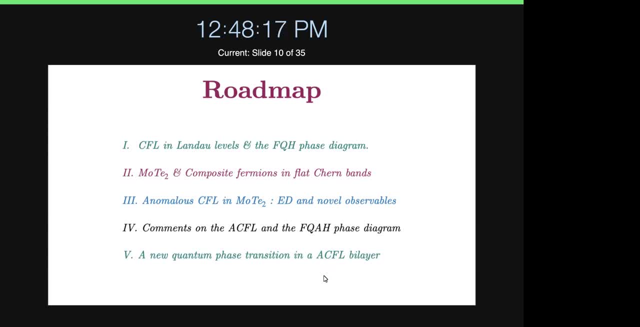 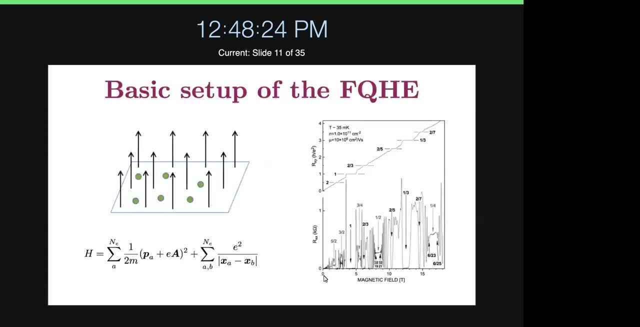 also the phase diagram of that system and make some final additional comments at time permitting. Okay, So some introductory feel about the fractional Hall effect First, we we all know that we just take a 2D electron gas in perpendicular magnetic field. 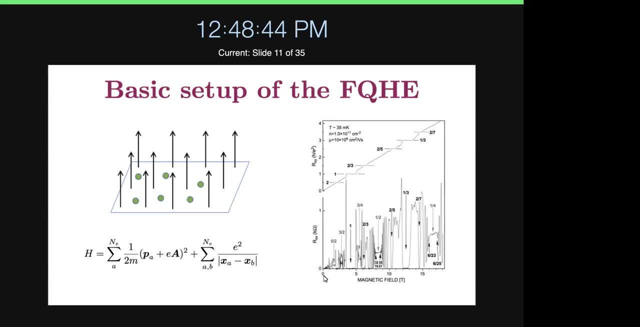 See that the electrons are going to form extremely highly degenerate Landau levels and realize when Landau levels are filled, phases with integer Hall response is the integer Hall effect And then, in the presence of Coulomb interactions, you can then get additional features here shown. 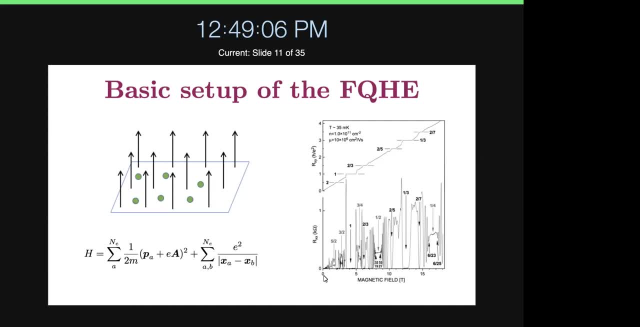 two-thirds, two-fifths and so on, And again, in addition to all that, you can see even denominator fillings here, perhaps more clearly than the previous slide, these composite Fermi liquid states. Okay, So composite Fermions. 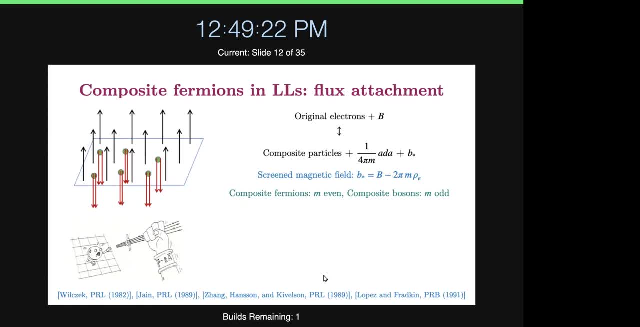 provide an organizing framework for all of this. I can start with my system of electrons as a field and always adiabatically attach fluxes to them to map my original system to a system of like we'll call composite particles coupled to an emergent. 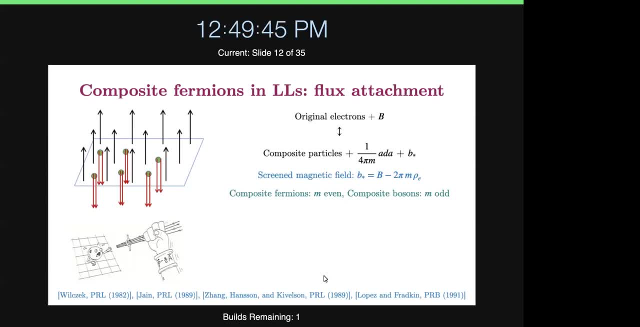 Chern-Simons gauge field and feeling a screened magnetic field where the screening is proportional to the density of the number of particles I'm attaching flux to And, depending on whether the expression is even or odd, I'll either attach an even number of flux. 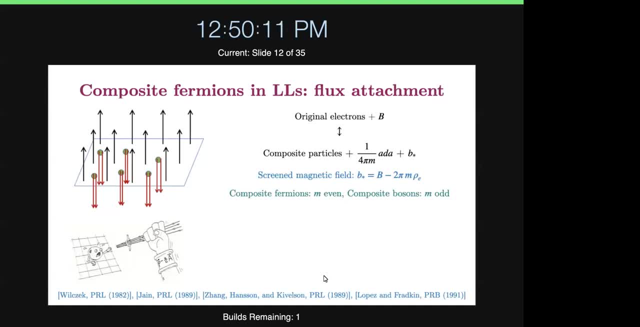 in which case the baryphase shifts by two pi. my statistics remain the same or not, baryphase? sorry, our own phase shifts by two pi. Or if I attach an odd number of flux, I'll get my statistics shifting by pi. 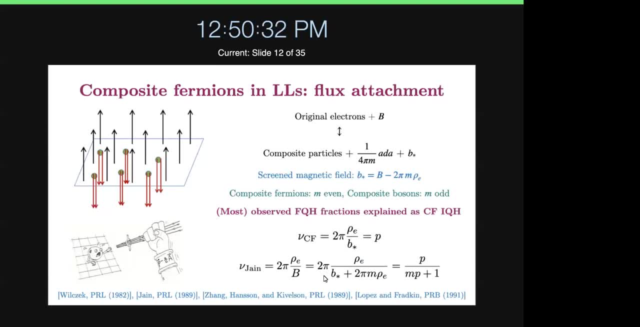 so if I'm going to focus primarily on the composite fermion case, it turns out that most observed fractional quantum Hall fractions can be explained as integer quantum Hall phases of composite fermions. So I start with, say, attaching two flux quanta I fill. 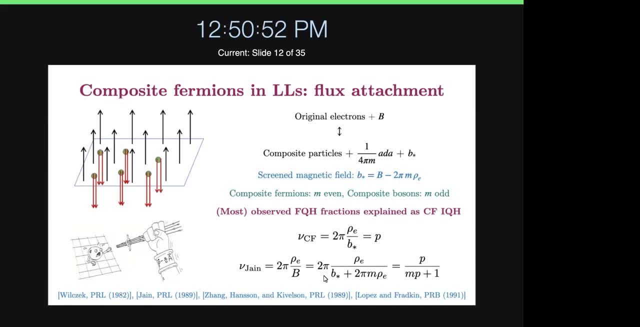 Landau level of these composite fermions by doping and I get. well, let's say I fill. I compute the resulting filling fraction of the electrons, I get the classic Jane sequence of fractional states, which actually describe most of the states that we have in. 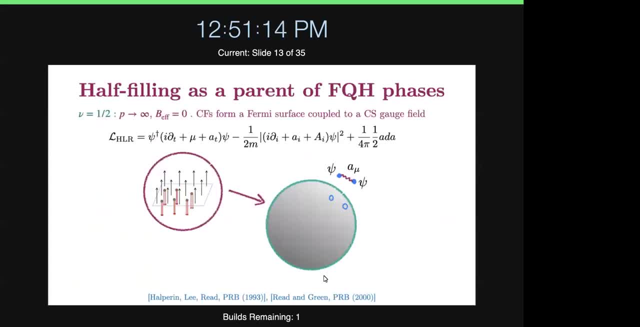 nature. Okay, Now if I look close to half filling. so this is like taking the limit as the effective magnetic field felt by the composite fermions goes to zero. a Fermi surface of composite fermions? Okay, because they, these are fermionic. 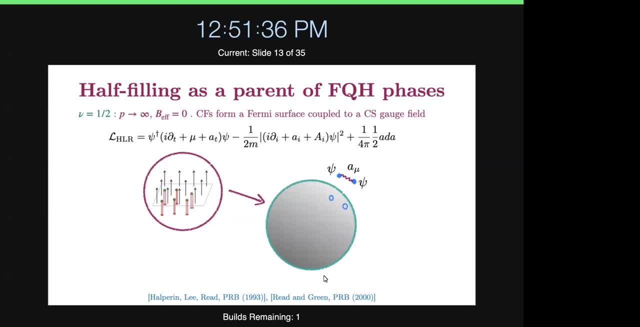 objects. they don't feel magnetic field. they're going to want to be a metal, but they remain strongly coupled to the subversion gauge field. This is the famous HLR theory of the half filled Landau level. Simplest, or it might be. 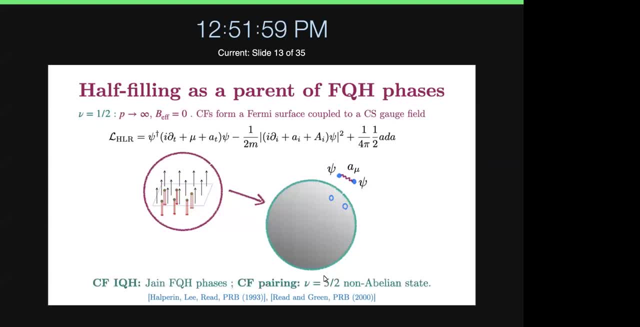 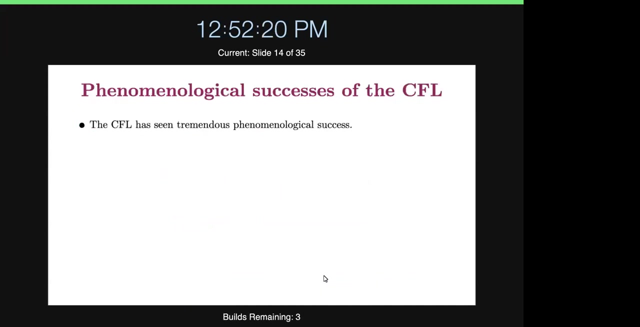 the simplest thing you can do And yeah, I said before, I just form all states of these things, get gene sequence states and also I can actually explain some non abelian states using these guys through parent. Now this composite theory predicts a: 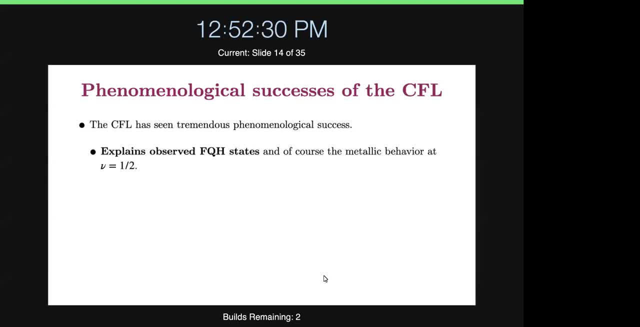 great deal more than just the gene states. It also explains quantum oscillation measurements. So one example is: I can introduce a periodic potential with some wave vector Q and I'll expect magneto resistance minima as I tune away from the current orbits or commensurate. 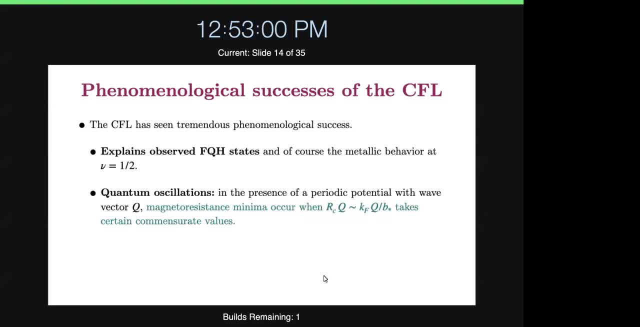 with periodic potential And actually this composite Fermi liquid theory beautifully predicts this kind of experiments: Modulo, recent, somewhat recent experiment that still people are working on explaining, But the vast majority of quantum oscillation measurements, in particular the realization of particle hole symmetry. 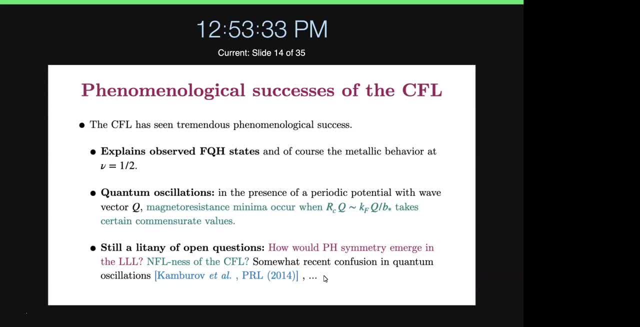 which is a problem that's been near and near to many of us for a while, and also questions related to dynamics of the composite Fermi liquid. What sense is it truly a non-Fermi liquid? Can you get non-Fermi liquid transport? 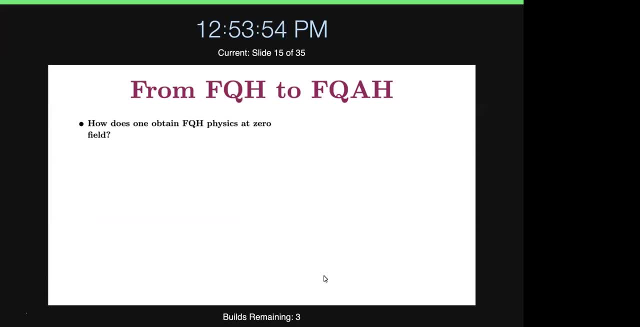 in something like this. It was ultimately a non-Fermi liquid, So now I want to take this physics and pour it over to zero here. So how does one actually do this? Well, you need a few ingredients. First, I need: 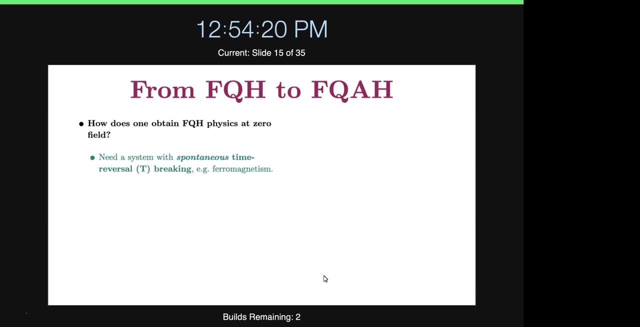 to get rid of time reversal symmetry without an external field. Yeah, the mic is, mic is on. so yeah, I don't mind the elections Now with this time reversal breaking one then would also need to form narrow turn bands. So these 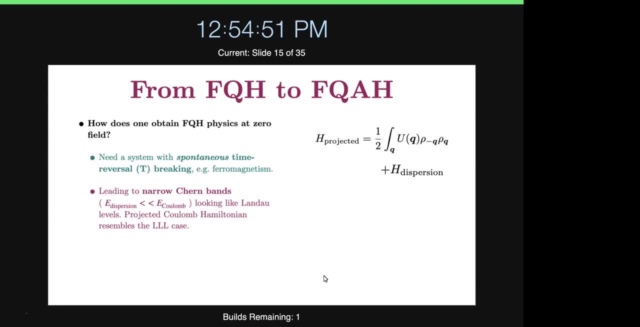 are fairly flat bands which are much smaller than the coolant energy And as a result, then, if you're sufficiently like a Landau level, the projected Hamiltonian which I've written here into the band will at least well resemble in their ways of. 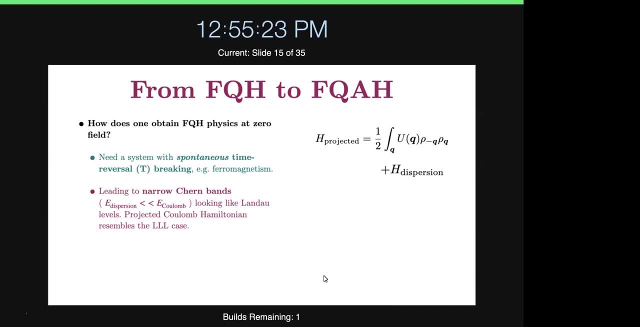 precisely characterizing this Projection in the lowest Landau level. So in the lowest Landau level case you just have, you have no dispersion, they're perfectly flat and you have ordinary coolant density interactions and the projected density operators satisfy what's. 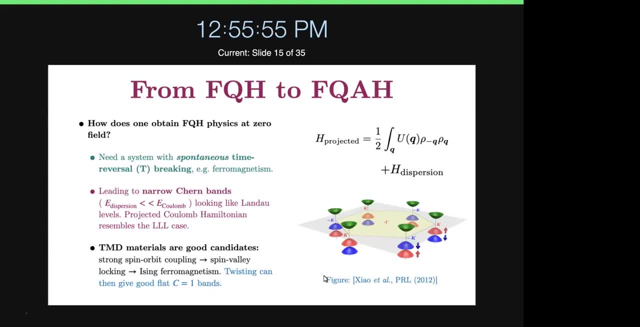 known as the Milita telluride system that I mentioned. I showed data from earlier in this talk are actually quite good candidates for both of these properties. So because of strong spin orbit coupling you get walking of the spin in valley degrees of freedom. 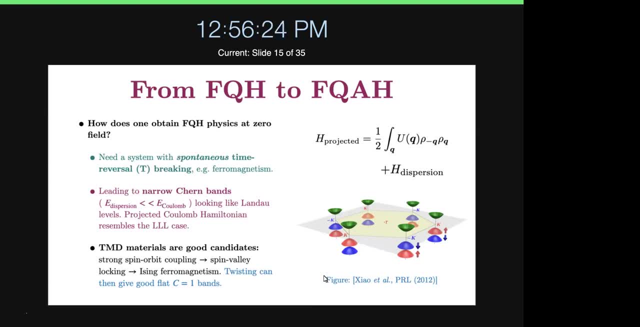 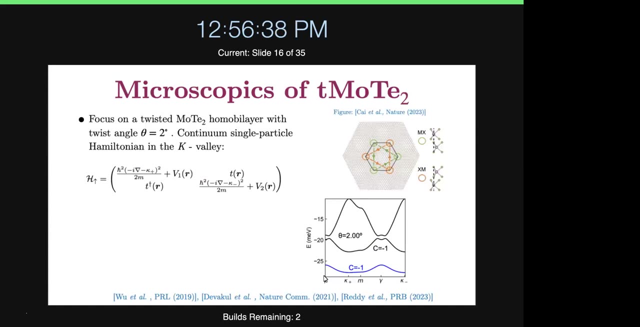 which provides twisting and displacement field. you can design a relative A-side plane. Sorry, there's a question. Okay, All right, so I'll explain briefly how we microscopically model this problem, So we can focus on the microscopics of a twisted molybdite telluride homo bilayer. 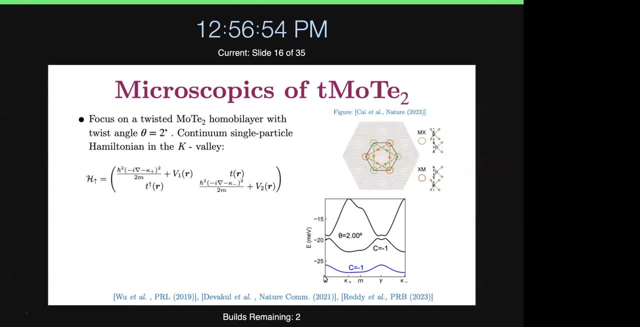 with twist angle set close to two degrees, And I can write down a continuum Hamiltonian for this that has been developed by other folks Here. these v's correspond to the moiré potential and the t's on the off-diagonal are the interlayer tunneling And we fit these parameters. 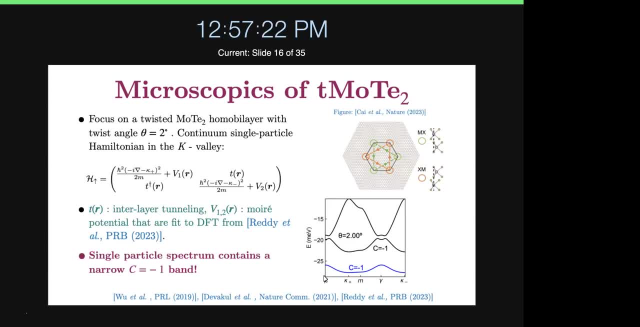 to results from DFT. So maybe one should mention that there was this other paper that I mentioned at the beginning of the talk that sees similar physics to us. They use different DFT parameters from the ones that we chose to use. That's awesome that with both sets of DFT parameters you see. 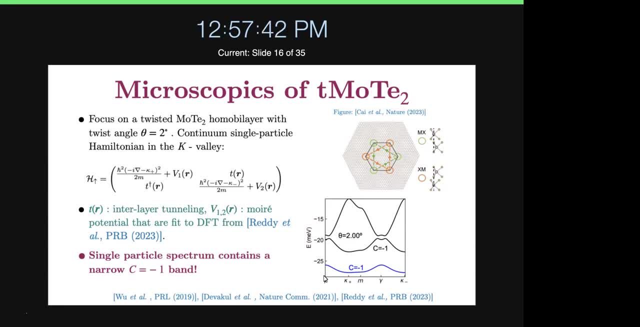 a similar physics, But in any case, the single particle spectrum that you can compute out of this thing contains a narrow C equals minus one band shown down here. All right, really, I keep saying down here to the folks at home, can't see my. 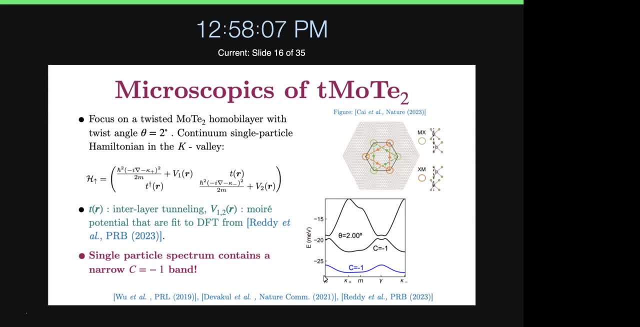 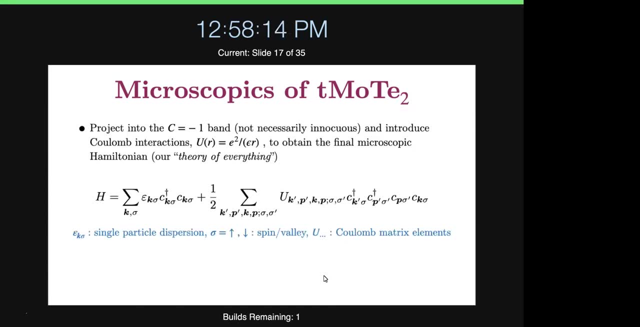 hopefully context one. All right, good, So now I can take this result and I can form a projected Hamiltonian into this band with Coulomb interaction. And this is the thing I'm going to be studying, not me, Aidan, who actually does the numerics. 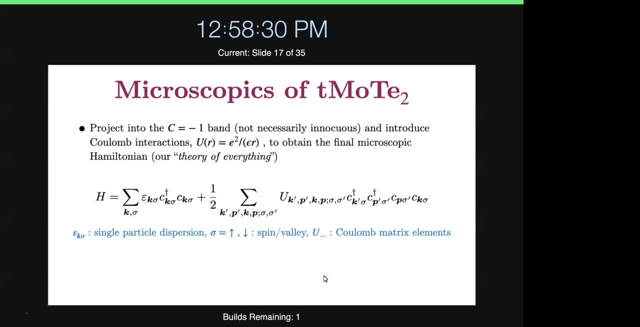 in exact diagonalization. So I have this first term here, which is the dispersion of the band, and the second term here is the interaction term, And I'm going to include spin and valley here, if you want to make sigmas, and 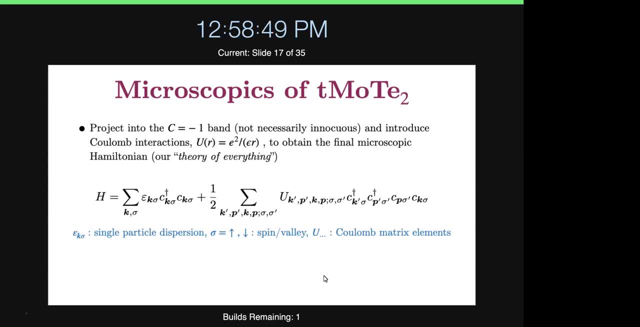 yeah, use the dispersion and Coulomb matrix elements I get from microscopic. All right, And you know, as I already said, we're going to study this Hamiltonian in ED. but I first want to motivate what the ground state properties are going to be by developing a 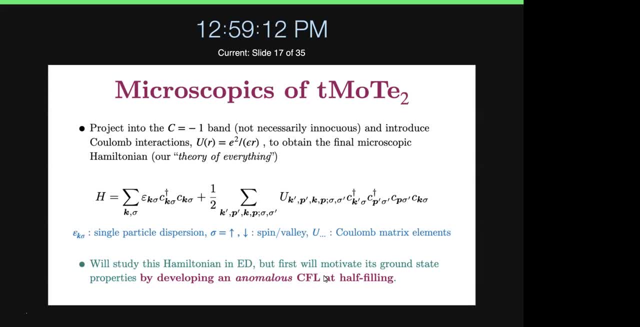 similar theory of the20-A-Milza-Fermian, a slide I discussed before in the context of a flux attachment in the Landau level. for the case of what I'm going to call for the rest of this talk, an anomalous composite Fermi liquid. So we can see the composite Fermi liquid: zero field. 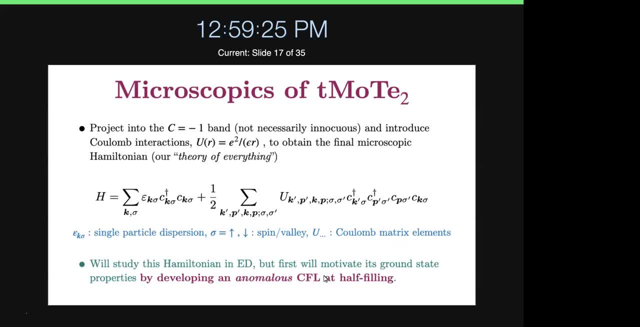 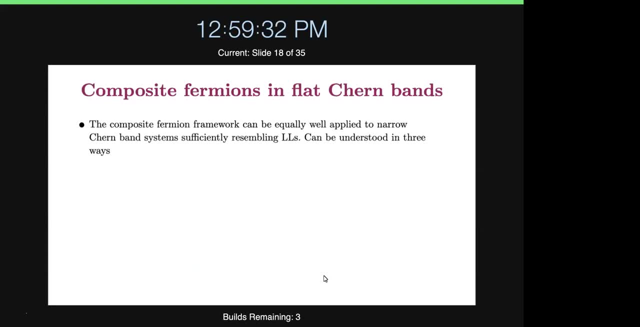 at half filling and then taking that composite Fermi liquid and we're going to dope it and form fractional non-Hall states eventually. All right, so we can try and construct the composite Fermion framework in churn bands in three ways. The first might be okay. we try ordinary flux attachment. but 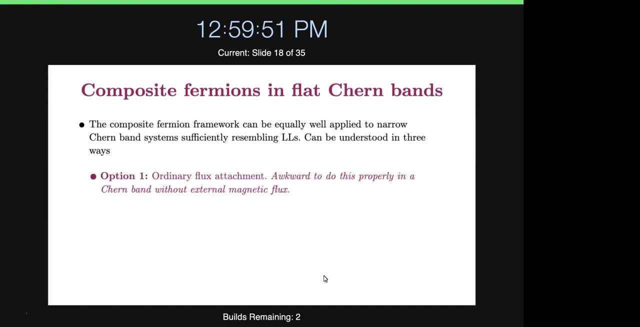 this is actually somewhat awkward to do in the context of a churn band. you don't have an external magnetic field. Theoretically, you can get the right answer with this, but in terms of constructing a systematic equivalent to flux attachment, it's certainly at least not. 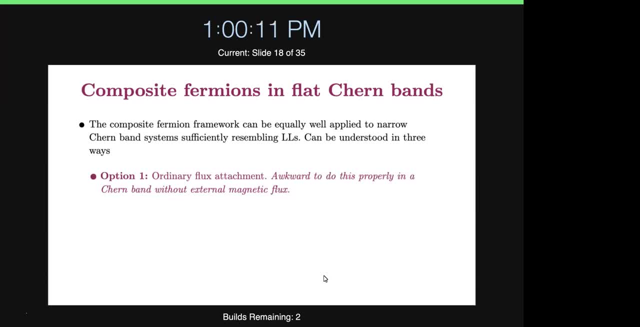 straightforward. There are analogs of lattice flux attachment that have been developed and those involve using lattice assignment theories and it's a bit of a. it's rather involved for especially for modeling real systems. Option two is to try to project into the churn band and 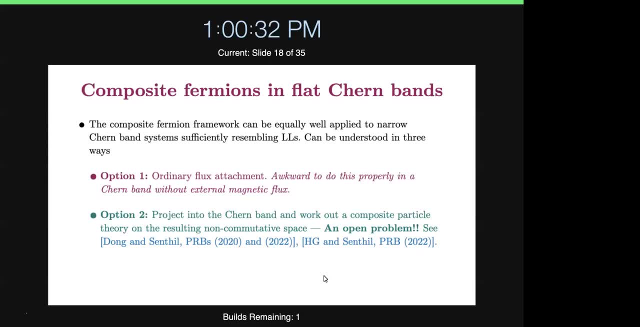 directly work out the composite Fermion picture in the non-communicative space of the churn band itself. This is a very hard, open problem. I can solve it in particular settings which are related to Landau levels, but certainly not this more general setting. but anybody who's 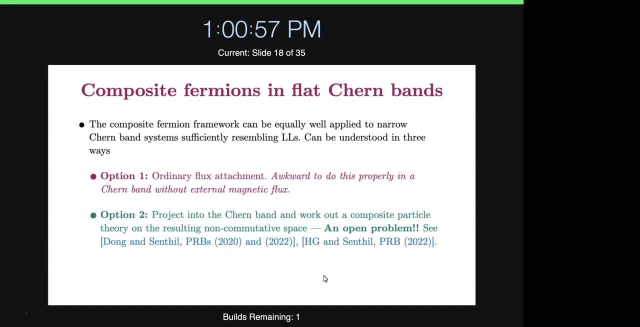 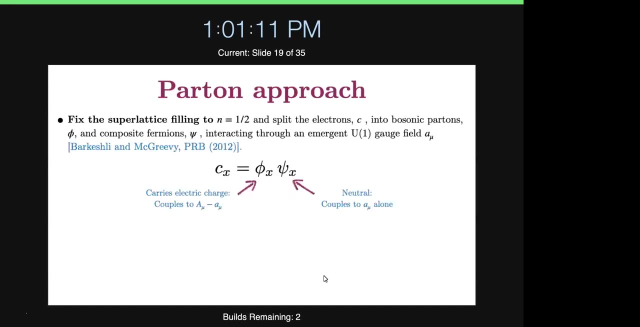 interested in this direction should feel free to talk to me or send me an email. It's a very interesting open problem. And option three is when, when in Cambridge you, as people in Cambridge, you do partons- Okay, so the parton framework has an advantage of well- you can generate tons and tons. 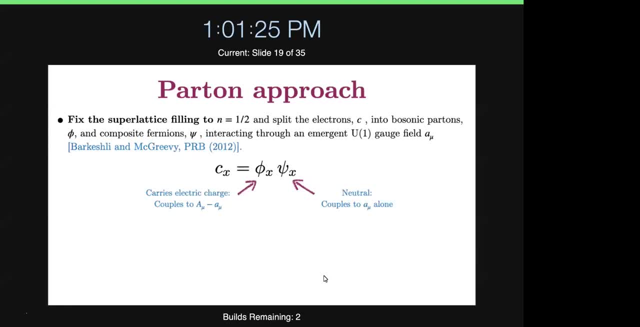 of states. with this, You can do it in fairly general band structures as a way of generating valid, effective fields. So I'm going to start with my Moiré superlative. So I have this filling. as n equals one half, I'm going to split the electrons which I'm denoting. 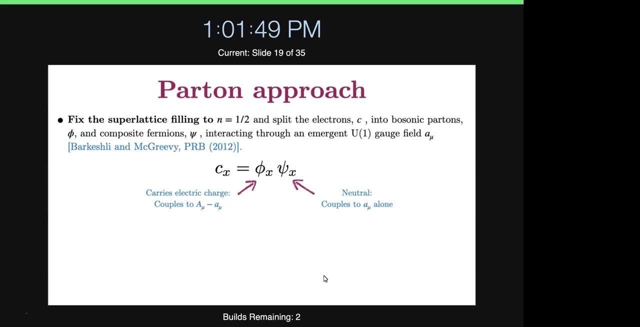 by c here into a bosonic parton phi and a well called composite Fermion psi, And I'm going to have this full on here. the bosonic parton carry the electric charge which I'm denoting by this background gauge field capital A. 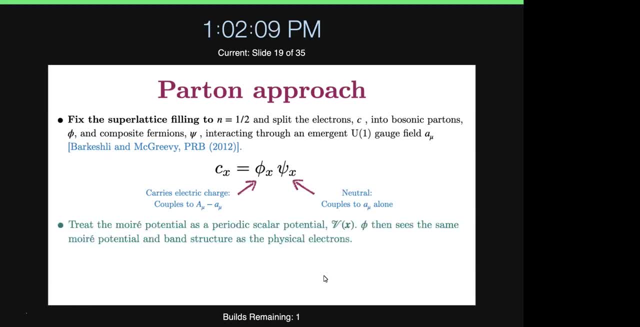 Okay, And I'm going to treat the Moiré potential as a periodic scalar potential. So in a sense I'm hiding it in big A and as a result of this, phi is going to see the same band structure as the underlying electrons and it's going to half fill. a c equals minus for the band. 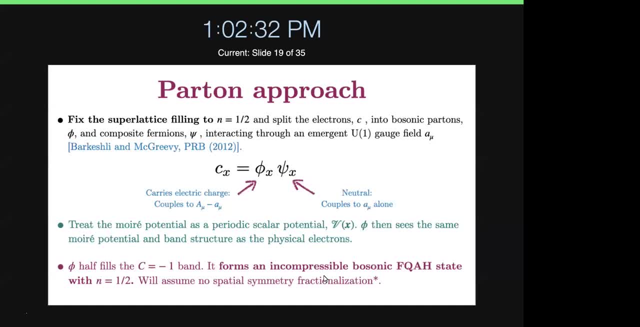 Well, that gives me a incompressible state. It's a bosonic Laughlin state. Add zero field and I can integrate out. Now, part of this involves making some statement about whether, about how, the spatial symmetries are realized in that state. I'm going to assume that they're realized in a trivial way. 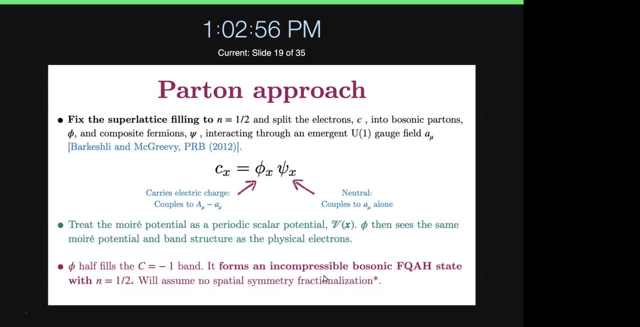 but that's not an absolute necessity and it's exploring the different kinds of possibilities for generating states with interesting symmetry. fractionalization from composite fermions is, I think, an interesting argument in that open direction that I and others are working on. So, okay, what do you get when you integrate out this phi? 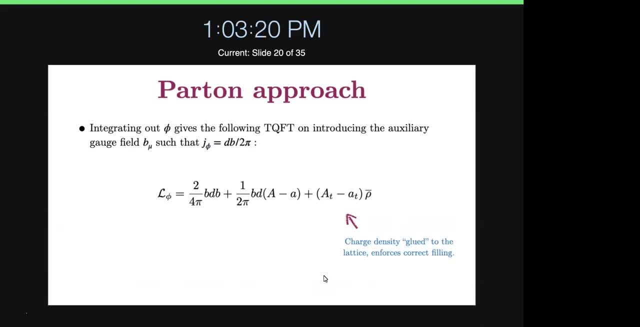 You get a TQFT which looks just like a bosonic Laughlin state. you have this Level 2 Chern-Simons theory, mutual Chern-Simons- second term, and then you have this additional third term which essentially fixes the filling for you without needing an external magnet, And you can think of that as like a charged nutrient. 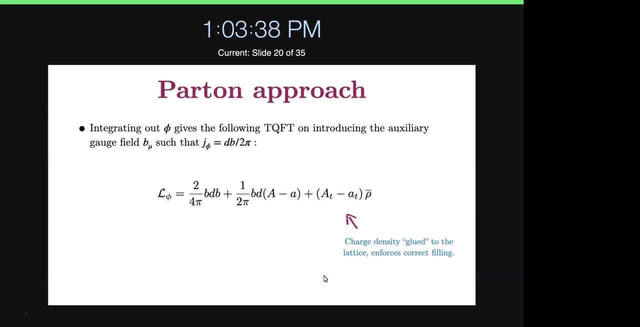 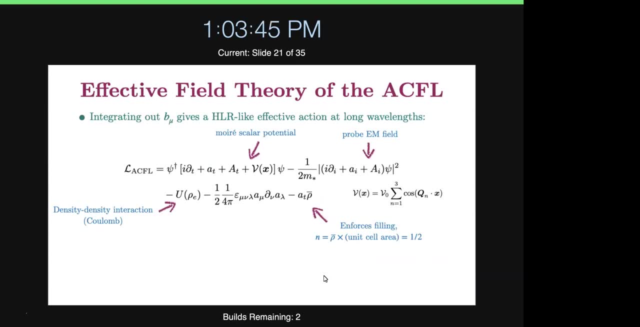 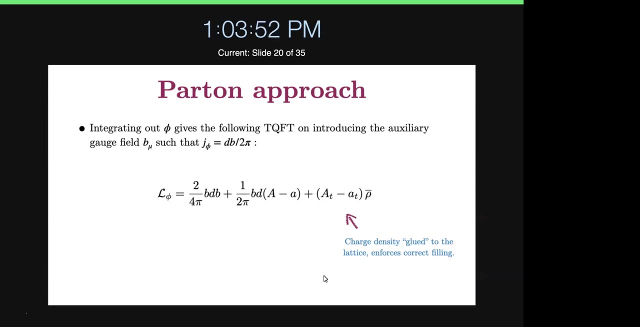 Okay, like a charge density that's glued to the underlying periodic bonds. OK, so I can integrate out this auxiliary field of B here that I got from integrating out the boson And you get a resulting theory which looks very similar to HLR. 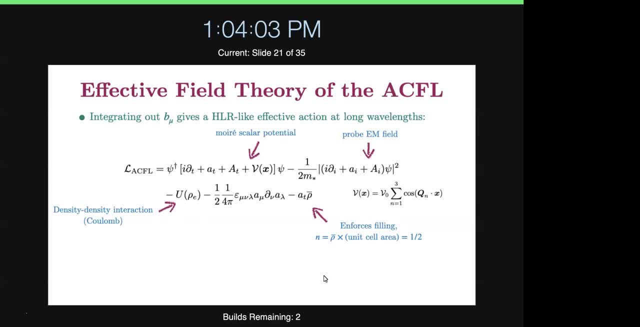 So the main differences with HLR are that I have this curly V here which models the Moiré potential, So it's a renormalized potential which will have the same period as the Moiré potential, And I will also have this term involving this row bar here. 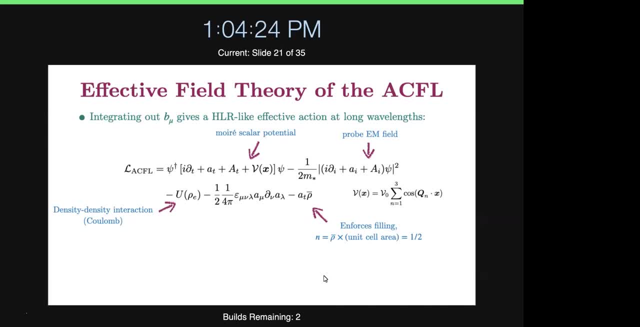 which again fixes the filling. And in particular, you can see explicitly how this fixes the filling by looking at the equation of motion for the time of the component. So little a which is, by the way, all these a's are U1 gauge fields, big A's are probes background. 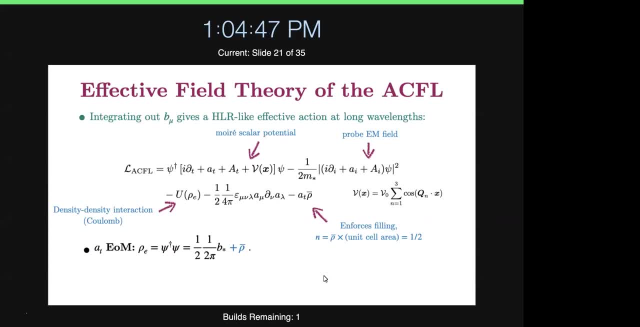 Little a is dynamical And, yeah, ASFT's equation of motion gives you a constraint fixing psi, dagger psi, which is also my electron density, to the sum of the emergent magnetic field associated with little a And row bar here. So when the composite fermions feel no magnetic fields, 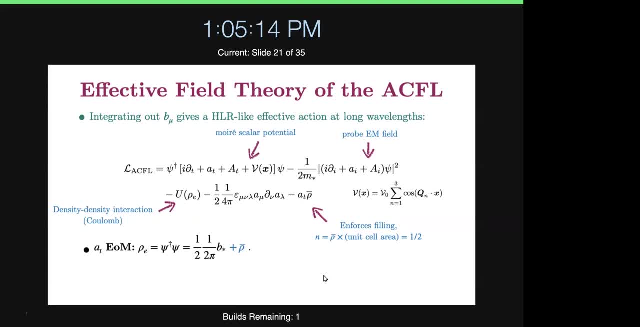 the b star is 0,, then the physical density is just and the physical filling is just the electron. And if I fix to half filling, then indeed the composite fermions feel no magnetic field, Form, what we call an anomalous composite. 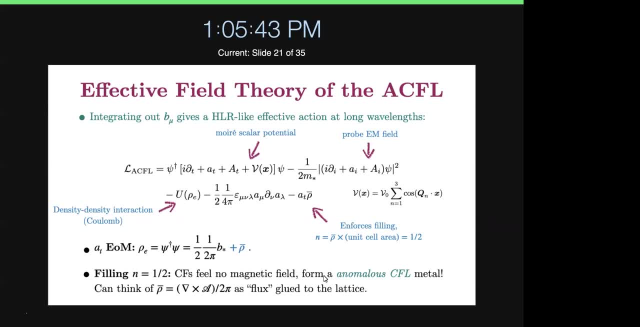 fermi liquid metal, And that again remarkably similar physics to the ordinary composite fermi liquid. Now I want to mention, if you'd like- I'm carrying this row bar around, but it's perhaps less mysterious if I rewrite it. 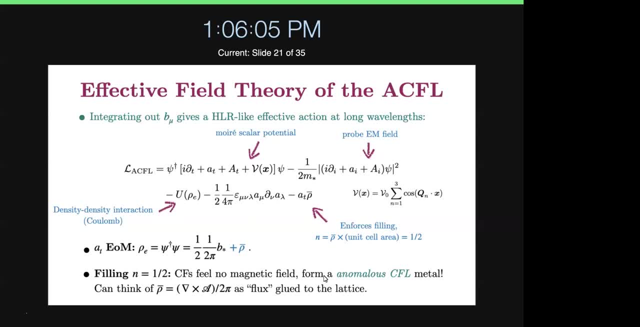 as the curl of some. So I'm going to go ahead and do that, And then I'm going to go ahead and do that, And then I'm going to go ahead and do that, And then I'm going to go ahead and do that. 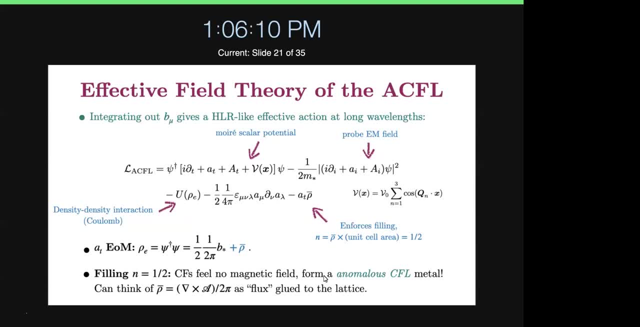 Background vector potential, which you can think of as being associated with the magnetic moments of this ferromagnetic state that I'm starting from. that breaks time. It's kind of a. that's a sort of heuristic analogy, which is why I emphasize using this notation, just using 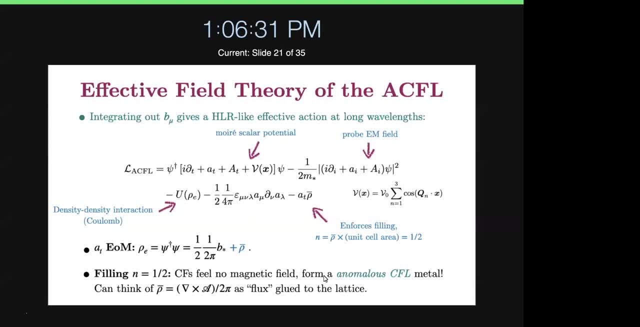 the row bar rather than a worksheet. Mutual terms, Simon's term, with chromium paint. Yeah, So in the part-time framework, is the n star equal to the bare mass or what the bare mass is? I would think that the gauge field is. 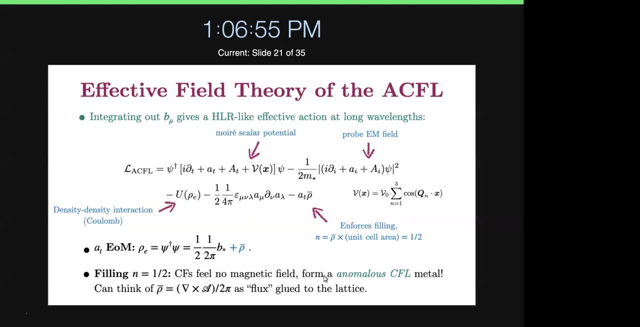 The gauge field will re-normalize this. So it's a question of- yeah, I guess, in terms of this, The part-time decomposition. technically, you only have the a0. That's right, And the ai gets generated Yeah. 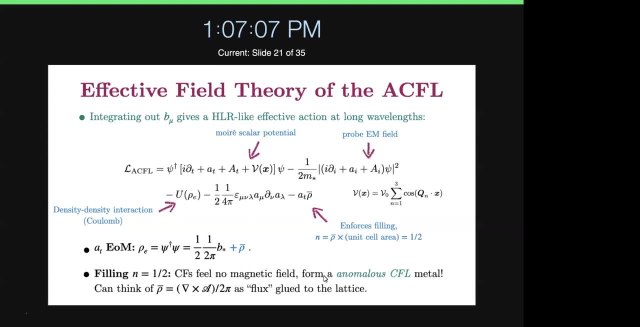 So it's. I guess it's a little different from the HLR, Like, say, say you do HLR for the ordinary fractional quantum polyphagy without a filling. If you just do the naive plus attachment versus part-time, you'll get different values for each one. 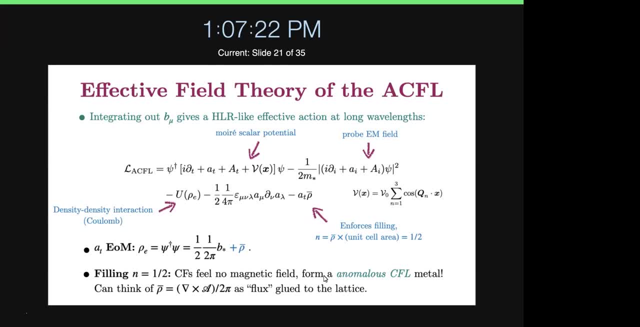 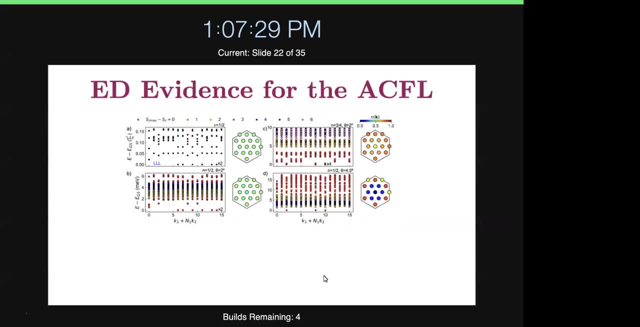 That's right. Yeah, Yeah, OK, Now how do we actually justify this beyond heuristics and effective field theory? Yeah, So we can do ED on a microscopic model I mentioned before And first get results that are actually amazingly similar. 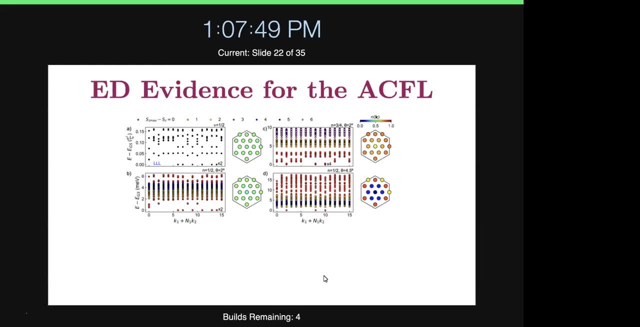 to the Haftel-Landau level. So we start by first looking at the Haftel-Landau level case. You get this ground state degeneracy here, So you just want to look at the bottom of these lots mainly. 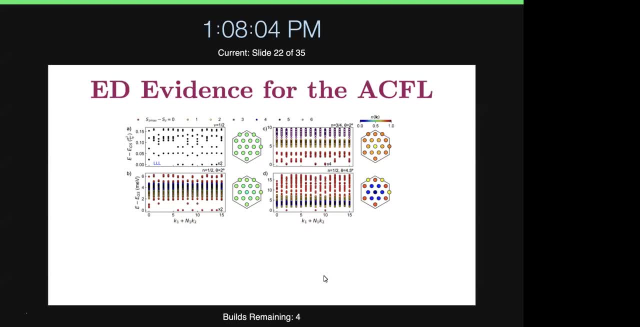 Then if I look at the Chern-Band case, that's going to look like this: OK. So if I look at the Chern-Band case that's modeled after moly-dietaluride, you get something that's very similar and match up extremely well. 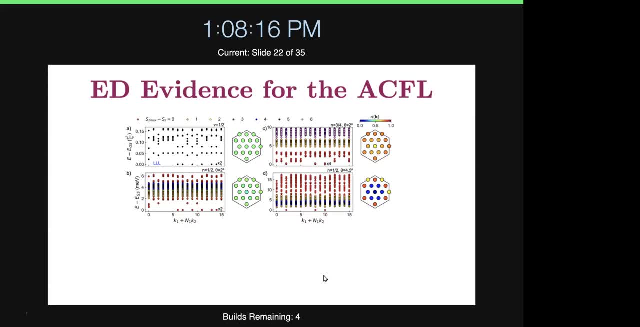 And you can think of these states as tiling a Fermi surface, the most compact Fermi surface I can write down in the Moiré-Broulant zone. So I fill center state and I start filling these states around here. 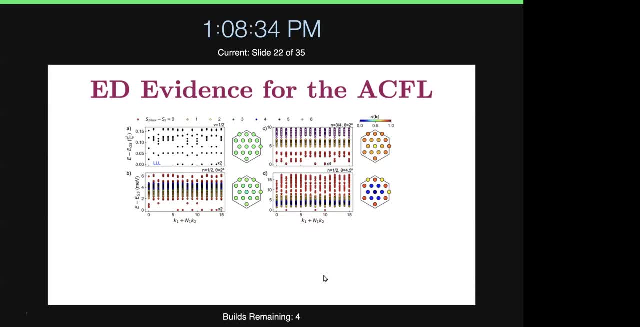 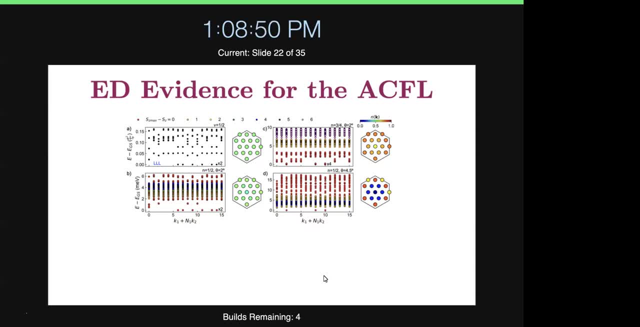 you notice they're all green. The reason for that is that these things are looking for the overlaps with log states. So what this is telling you is that you have this metallic state which does not have any overlap, with some overlap, but it's very small overlap with a metal. 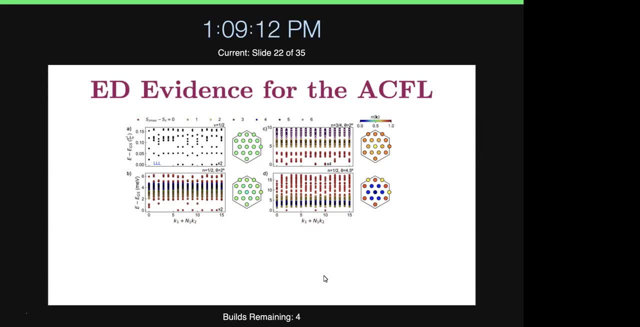 formed to block electrons. In contrast, if I change my twist angle from 2 degrees to 4.5 degrees, my bandwidth gets less narrow And I actually get a state that looks more like an ordinary Fermi liquid metal, in the sense that I just fill up. 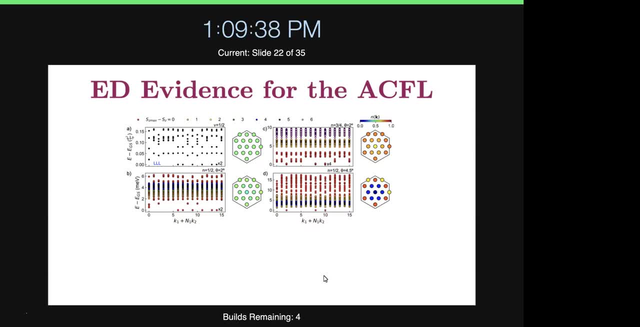 So the band minima are actually on the edges here. Red denotes a large occupation And I just fill up the edges of the Brillouin zone. I'll get to this top right corner here in 3 fourths and a second. So there's some comments on some of the specifics of the ED. 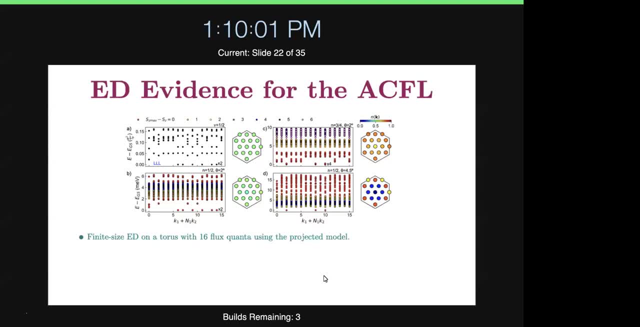 We did find Size ED. Aiden did find size ED on a torus with 16 flux quanta using the projected model from before. I already said this, Already, said this Now, yeah, I also want to emphasize that again. 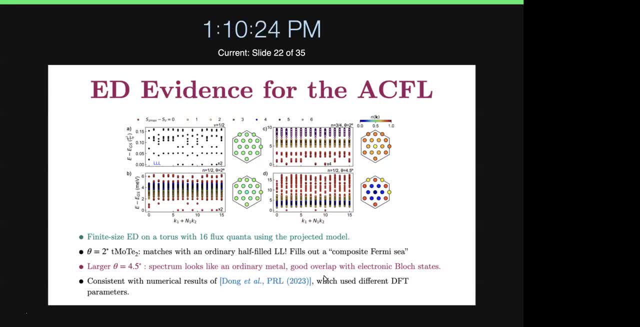 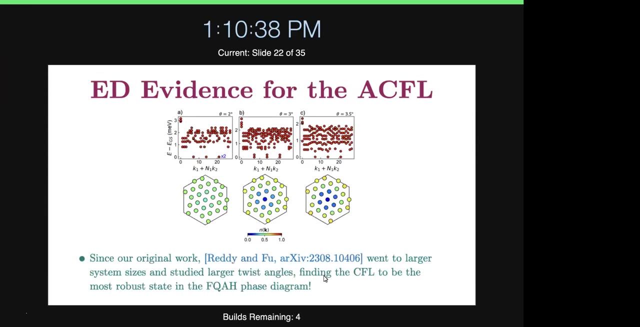 local people also did similar type of ED analysis using different DFT parameters and got very similar results. They also did amazing de-emerging. We didn't do de-emerging, OK. So now I guess I'll comment first on the 1, fourth state. 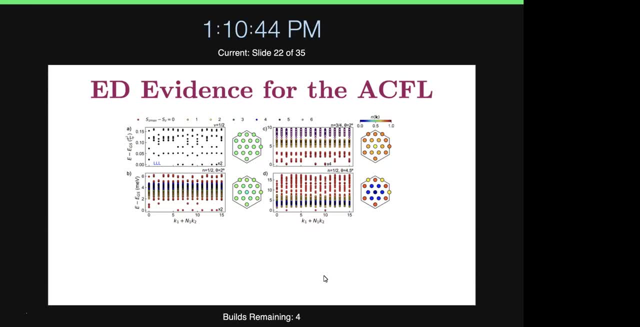 So you can also play the same game with the 1- fourth state Or not 1 fourth, 3 fourth state and see similar composite features. So you can match this with the Landau level and 3- fourths And actually, I think, the matching of the spectrum. 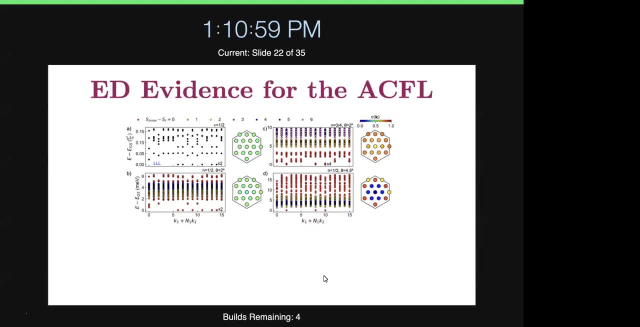 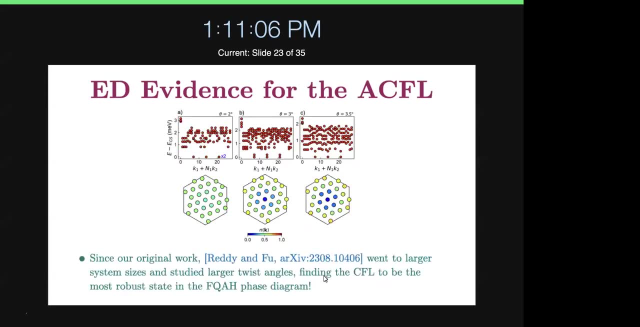 looks even better. Then, Yeah Yeah, The matching of the spectrum for 1 half. I had a slide showing that, But maybe it's actually after the next slide. OK, So now, since this original work, Aiden and Liang- 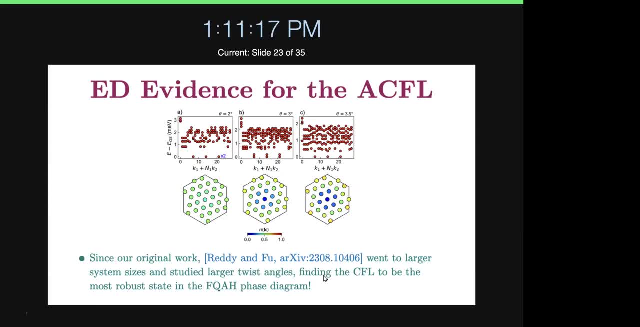 have been able to slaughter this problem at even larger system sizes and find, amazingly, that the composite Fermi liquid is extremely robust. You can go to twist angles where other Other Fractional home anomalous Hall states all die, But the composite Fermi liquid stays alive. 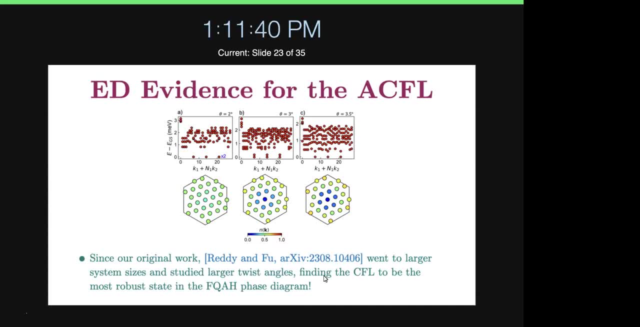 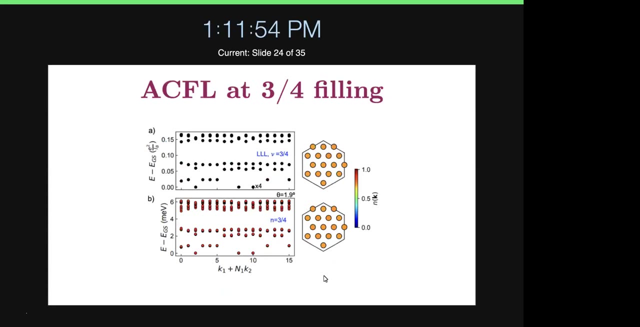 That's crazy. So, yeah, it really emphasizes the centrality of the composite Fermi liquid to the FQAH case. All right Now. OK, yeah, there's a slide on 3 fourths. Yeah, so you can see the matching here for the 3 fourths case. 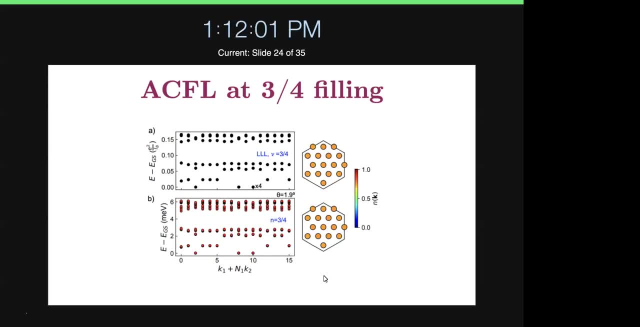 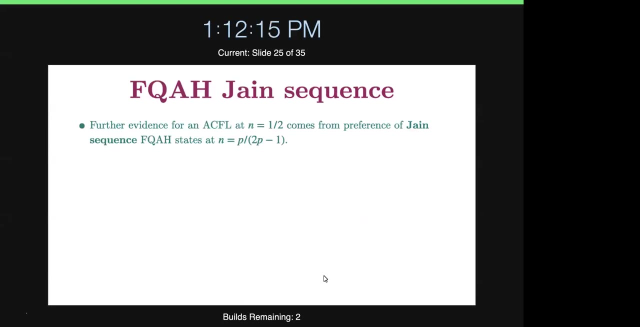 OK, So this is the difference between the lowest Landau level spectrum and the actual spectrum for the Moiré case. And you see, actually even the excited states match on each other pretty well. All right, Now I can play the usual game of generating. 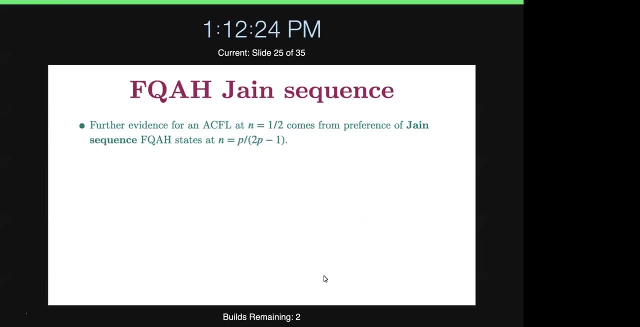 gain. sequence states using this composite Fermi liquid by filling Landau levels. And I get the usual prediction. Now one anomalous Hall states a 0 field at these filling fractions, the usual Jane ones. n equals p over 2p minus 1.. 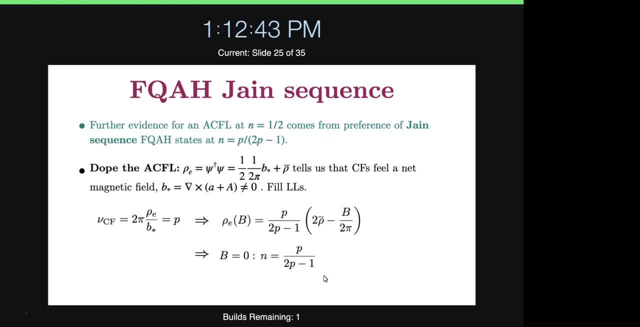 OK, so just the mechanics of how I do that can say: dope the ACFL by changing the electron density. Now the composite Fermians will feel a magnetic field and fill Landau levels And this results in the electron density. And the result in electron density when I filled p Landau. 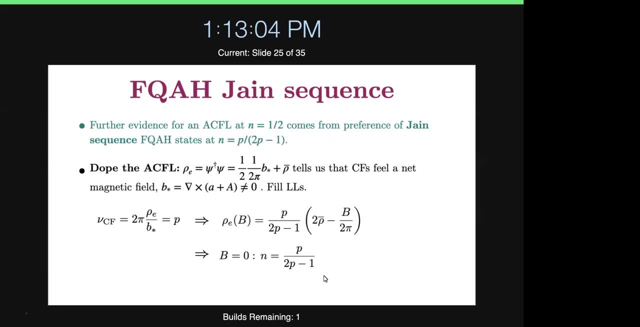 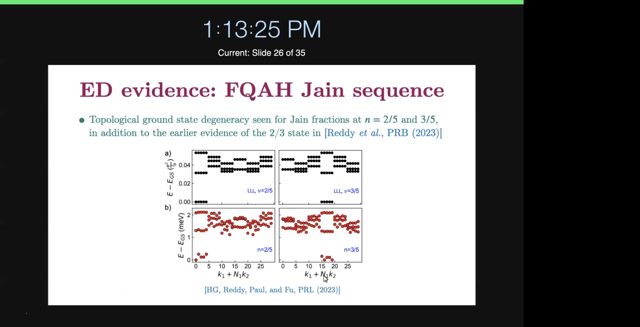 levels of composite Fermions equal to p over 2p minus 1.. And, as in the ordinary case, you can think of the composite Fermi liquid equivalently, as the p goes to impending limit of the Jane sequence states. All right, so we can also do ED looking for the Jane sequence. 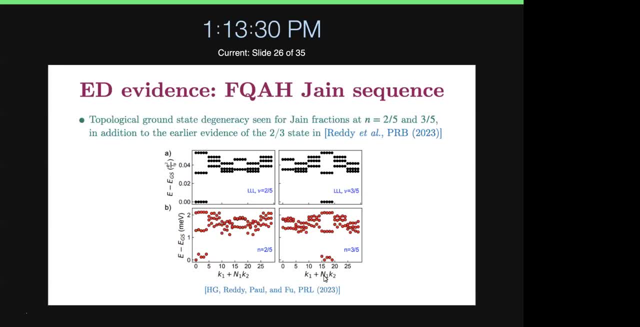 phases And you can see that they're very robust. That's further evidence for the composite Fermi liquid. You see robust states on the Jane fractions. That's giving you a hint that the parent of all these guys is the composite Fermi liquid. 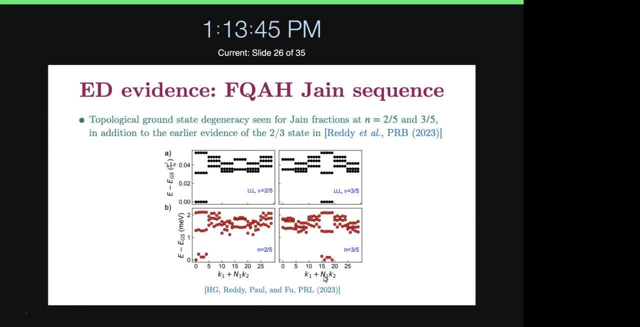 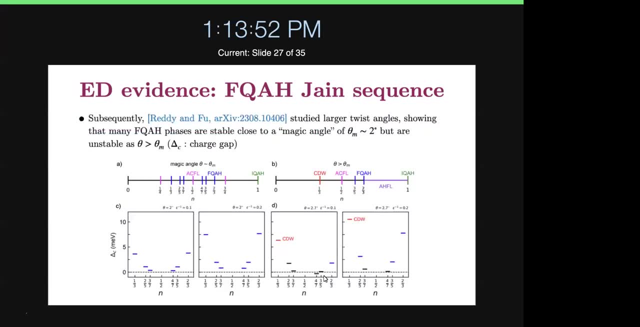 And so here's some evidence for 2 fifths and 3 fifths. You see the right topological ground, state degeneracy of 5 here, But amazingly now even can go to even more states and more twist angles and see all kinds of fractions. 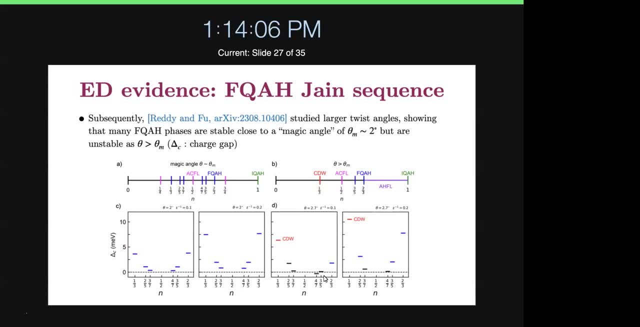 So here are the gaps depicted for two different twist angles. One is 2 degrees, The other is closer to 3 degrees, And you see that for the 2 degree case you actually get gaps opening up in ground states that correspond to several Jane sequence filling fractions. 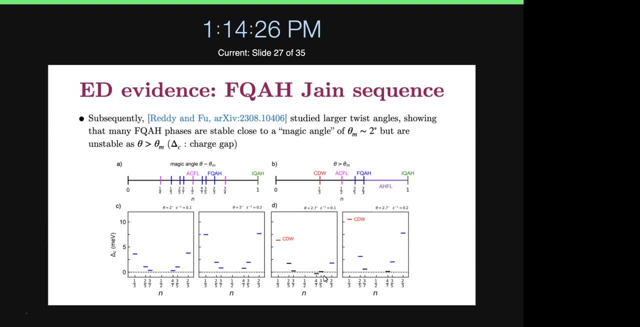 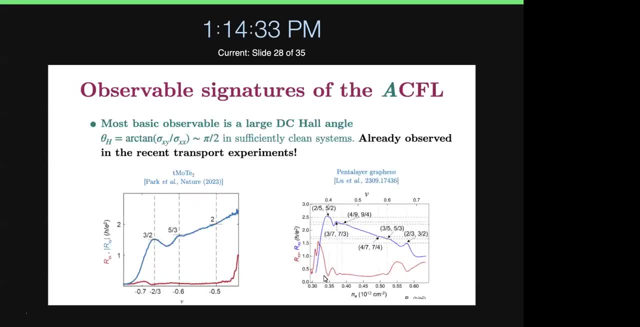 Whereas at larger twist angles these states will become unstable to things like charge, density, wave order or metallic features. OK, so what are the actual experimental observables associated with composite Fermi liquid beyond just Jane scales? So the first thing is that in sufficiently clean systems, 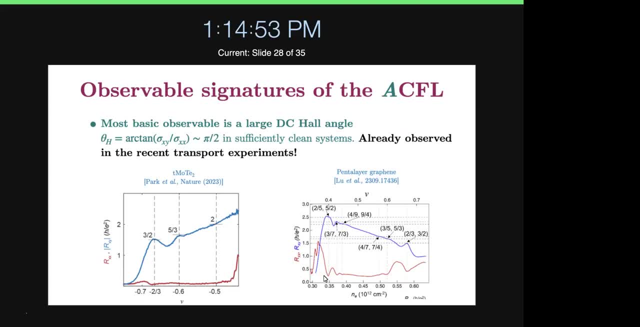 this is really the most stark thing one can look for is a large DC hauling OK, and that's actually already seen in recent experiments. So you see this haul conductivity near half filling, or haul resistivity near half filling, which is close to 2h over e squared. 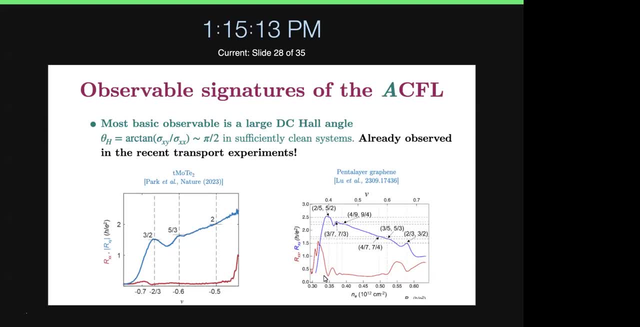 Whereas the longitudinal resistivity here is quite small. This is in the MOT2 case. In the pental layer graphene case it's a little bit worse, But it's still. the haul angle is still quite large. Now that's not a smoking gun for the existence. 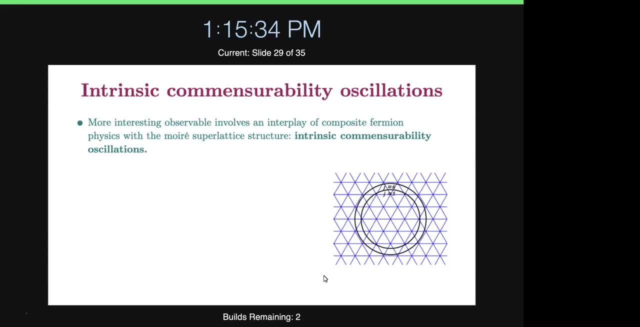 of a composite Fermi liquid state. When you have a metal, you should see quantum oscillations, Something that is unique about this anomalous composite Fermi liquid state, as opposed to an ordinary composite Fermi liquid in, say, gallium arsenide. 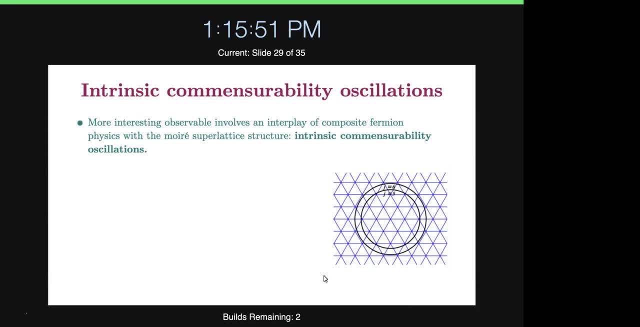 is, I have this periodic potential built in, So I don't need to add anything else. in principle, to see quantum oscillations, I can just tune the density which causes the composite Fermi on a cyclomagnetic field and look for commensurability oscillations. 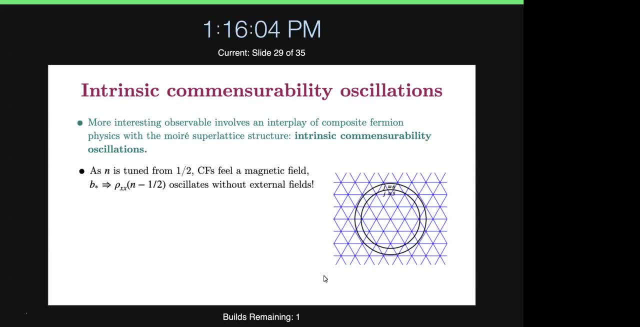 with the underlying where it is. So yeah, as I already said, if I tune away from 1 half with no external fields at all, I should be able, in principle, to see quantum oscillations And, in particular, find resistance minima where. 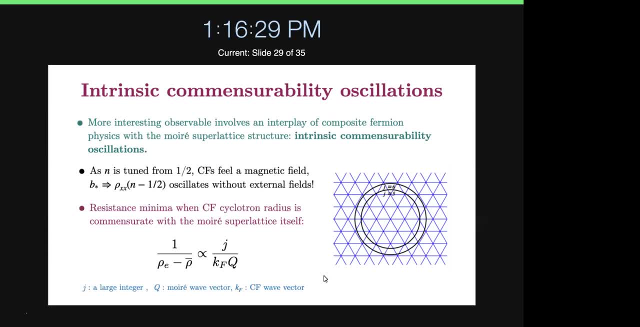 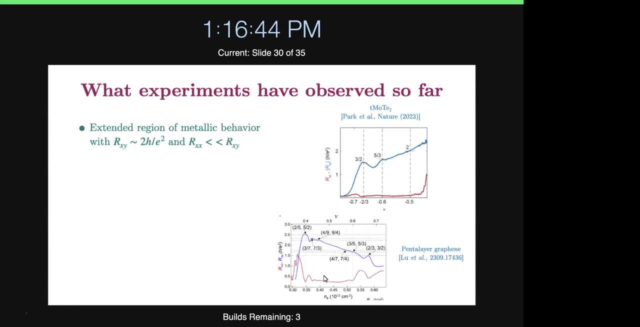 which is set by the Fermi wave vector and the Moiré superlattice wave vector. OK, good, So I already alluded to some of this, but I just want to emphasize what experiments have actually been seen. So first, an extended region of metallic behavior. 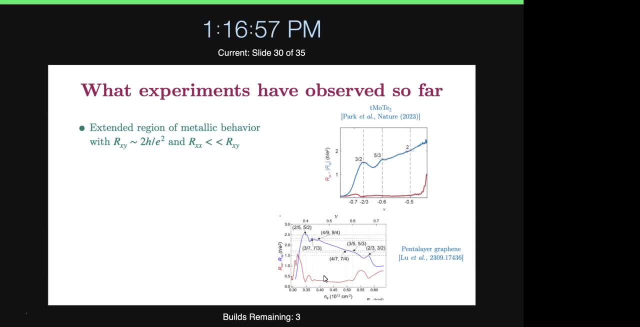 has been seen: close to Half-filling, with all resistivity close to 2, and Rxx reasonably less than Rxy, See the Jane sequence or the beginnings of the Jane sequence, And something that's not yet seen, though, is these commensurability oscillations. 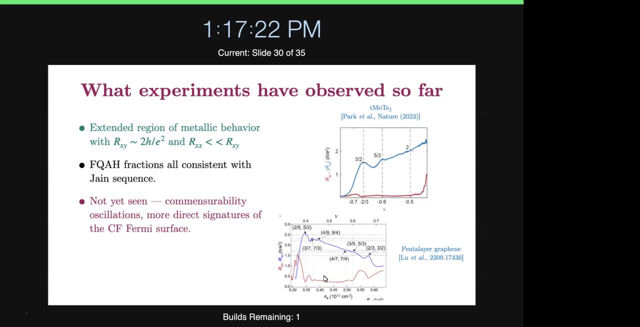 or more direct signatures, And that may require much cleaner systems. Now I also want to emphasize some additional features in these resistivity plots that are not immediately explainable by the ACFL In particular. one example is if you look at the transition from, say, the 3 halves. 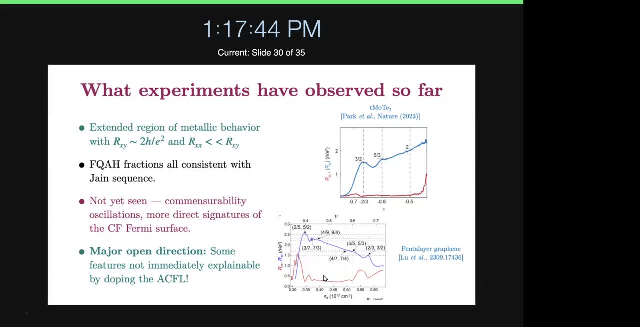 sorry. 2 third states to the 3 fifth state. you notice that the Hall resistivity drops between these two states. That's rather unlike anything that we see in OK. Normally we would have expected something more like a plateau, or at least an increasing Hall resistivity. 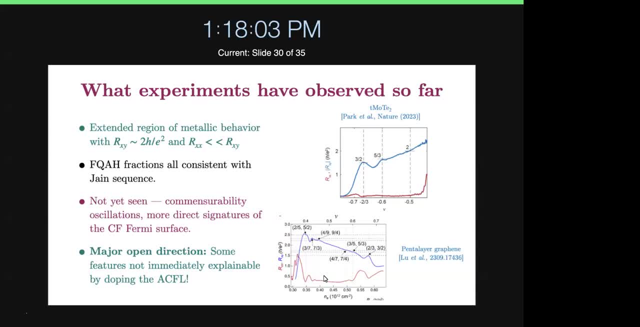 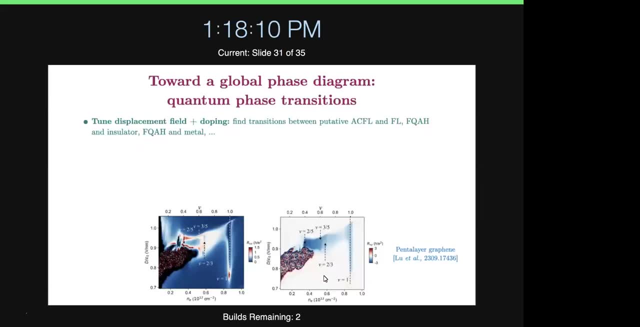 rather than decreasing. Understanding this in terms of doping, a composite Fermi liquid is still an open problem. I think it's a very interesting one. All right, So now I'll comment a little bit more on phase transitions. So, as I mentioned at the beginning of the talk, 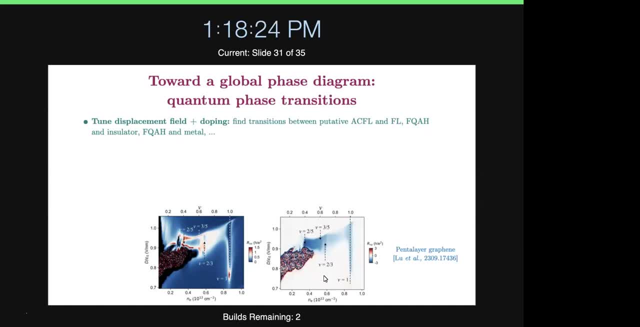 we now have this additional axis of displacement of fuel And that can in principle tune us between all kinds of different things: Composite Fermi liquid and Fermi liquid, which has already been observed experimentally, can get a fraction upon all the insulator fraction upon all. 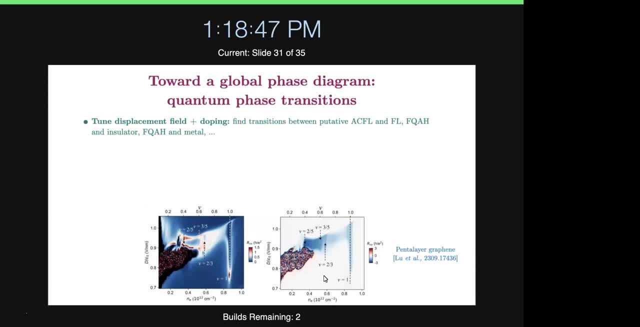 the metal, your favorite combination of things, And even if they're not seen, you can, in principle, think about these types of transitions. Now, However, only some of these types of quantum phase transitions are explainable using standard part time techniques, in particular the composite Fermi liquid. 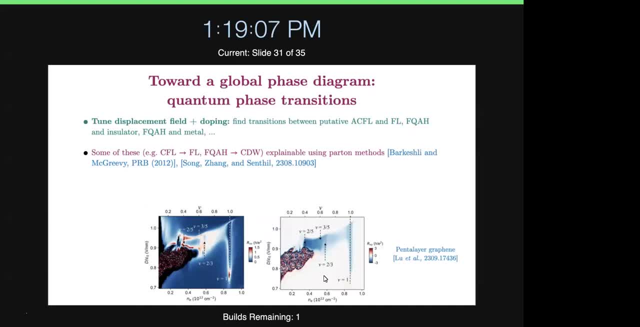 to Fermi liquid transition and the quantum monomolecule to Cw transition. But some of these features are actually quite unexpected. So even in the experiments there are signatures which, sorry, it's hard to point at these things. but 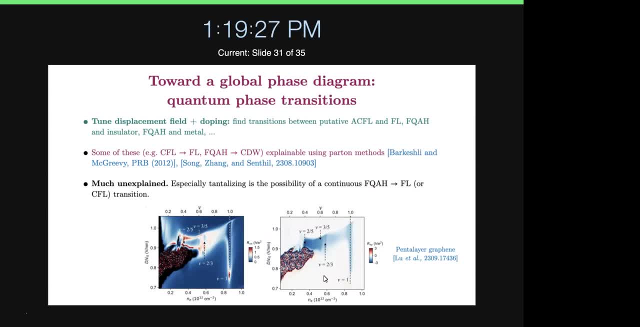 If you look, say, near filling 1, here there's a turn insulator And as I tune displacement field, you see that there's a little bit of an increase in the resistivity that would indicate the onset of metallic behavior. 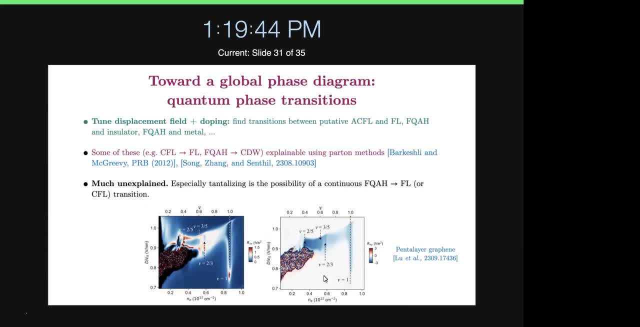 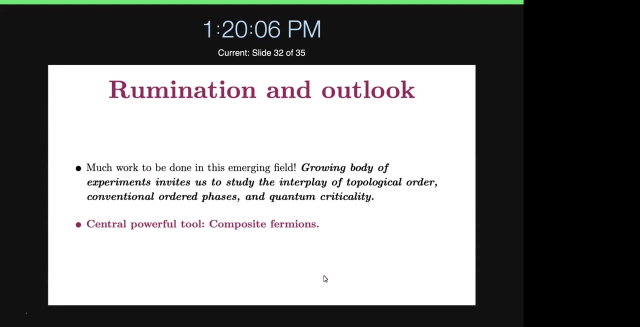 And you can see similar things for the fractional states. That indicates the possibility of something like a quantum anomalous Hall to metal transition, for which there's no theoretical foundation. That's an extremely interesting and important open question. All right, So before I conclude, I just want to say that I found all this extremely amazing. I 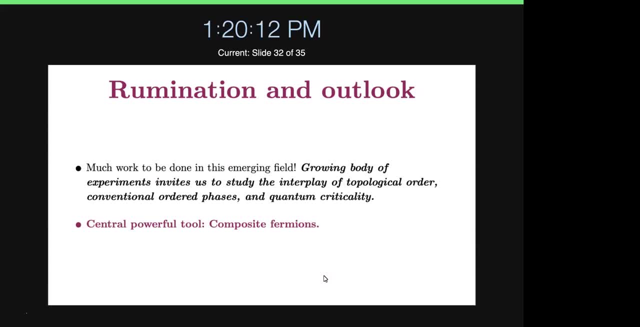 think that it's rare to see experiments like this that show us things that we know and also things that we don't know, And I think this whole field invites us to think about an interplay of correlations and topological order and different types of quantum criticality. 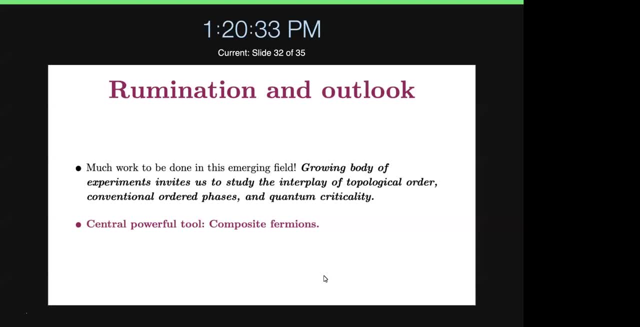 that hasn't been seen in an experimental set in quite some time. So with all of this, unlike usual mysteries and strongly correlated quantum matter, we have actually clear conceptual tools coming from quantum all physics, in particular composite variance. Okay, And for many future directions here, silk rowing in the field is. 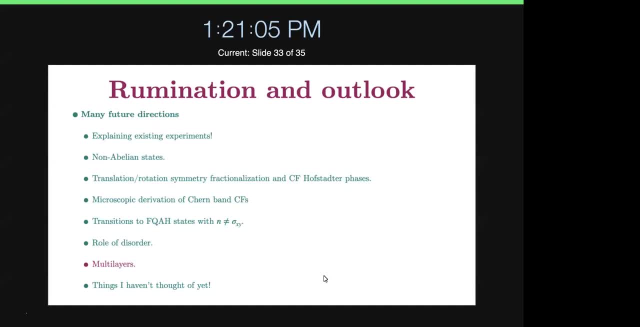 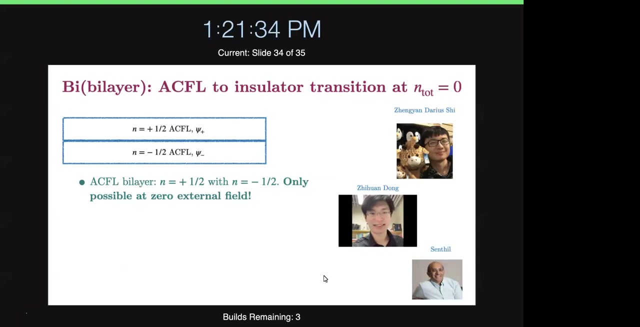 rapidly growing, where experiments will lead to even further things. But in my last few minutes comment on one particular additional avenue, which is dreaming of multi-layer Systems that are not realized in a finite field and exhibiting novel types of quantum criticality. So this is work with different people that will appear, hopefully. 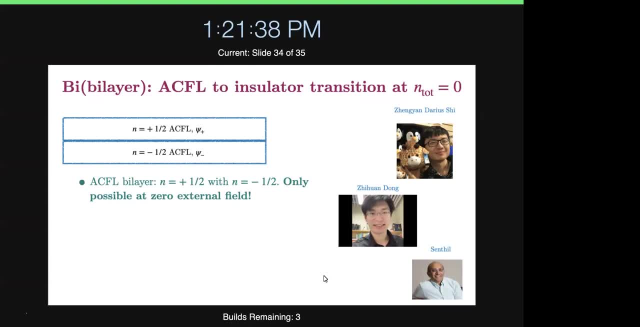 in the next couple of months. Darius is in the room. These other two apparently declined to show up. but thank you, Darius. But you start with bi-layer Now composite Fermi liquid at zero field and it's time-reverse conjugate. So imagine you have. 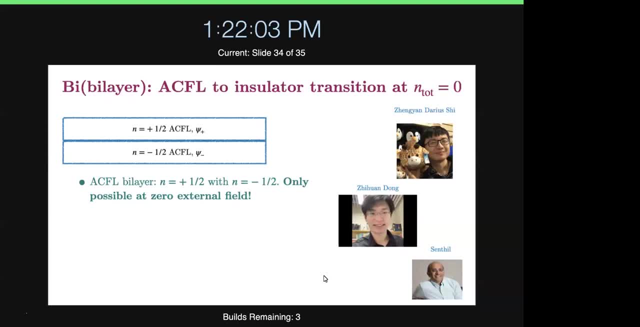 one magnet pointing the up direction, the other pointing the down direction, and you put them together and both are realizing this phase of the Bell state. So this is of course not possible. if you were trying to use one of all multi-layers, You would. 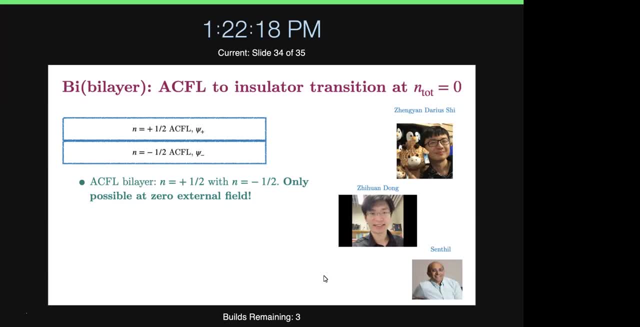 have an external magnetic field, You wouldn't be able to do something like this. Now I can try and couple this to an order parameter which pairs composite Fermions with what we'll call composite holes between these two layers and actually generate a non-Fermi liquid or composite Fermion. 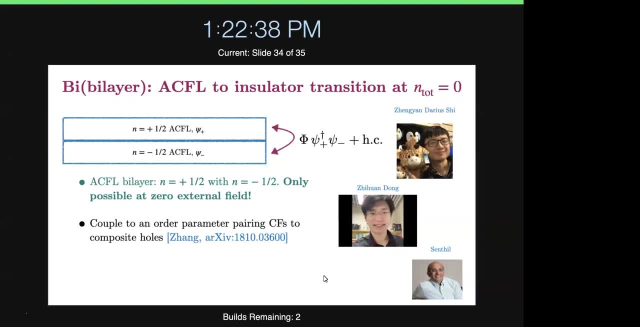 metal to mod-insulator transition, or what I'm calling a mod-insulator transition with a neutral Fermi surface. So that occurs when this phi, here this order parameter field, condenses. So why might I be interested in something like this? 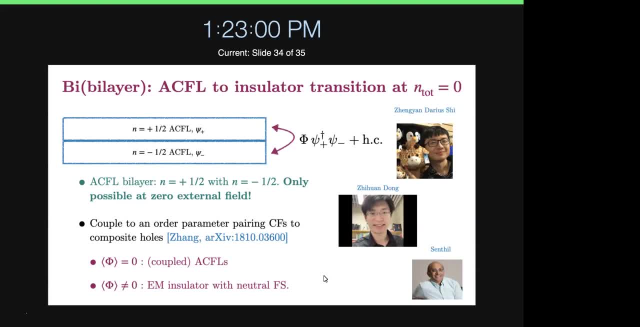 I guess I could imagine trying to set something like this up. We're working out the details of what might be a realistic experimental protocol, but I can at least think about this in theory space. It's a CMSA talk after all, So I could imagine say: 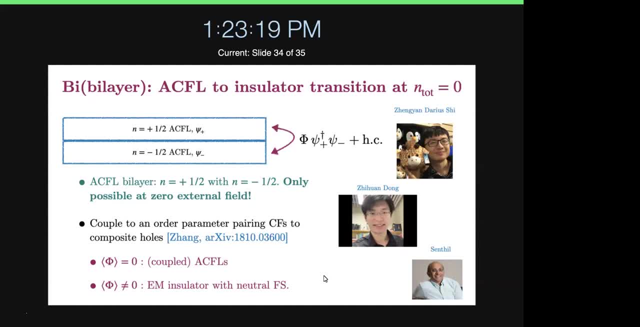 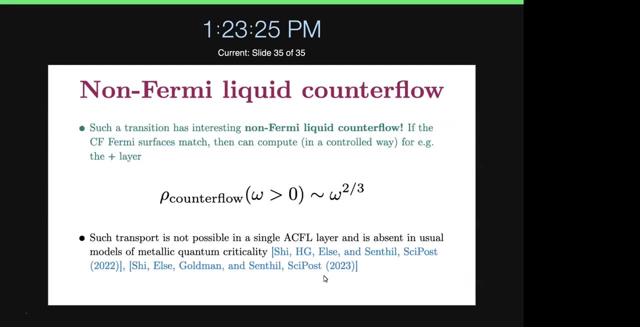 trying to change the distance between these two layers to tune this kind of transition. and the cool thing about this is that at the critical point you actually get non-Fermi liquid counter flow. So if I compute the optical resistivity I will see non-Fermi liquid scale. This is actually really hard to find. 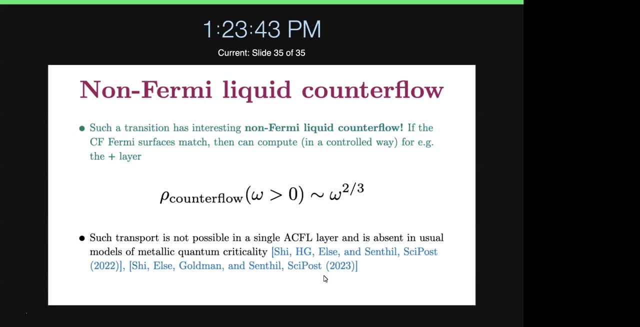 in transport in HLR in just single composite Fermion. But in the context of this particular example this ends up popping out rather naturally, at least with some calculation. This can be shown in controlled calculations. So that's going to be upcoming work. I should emphasize here. 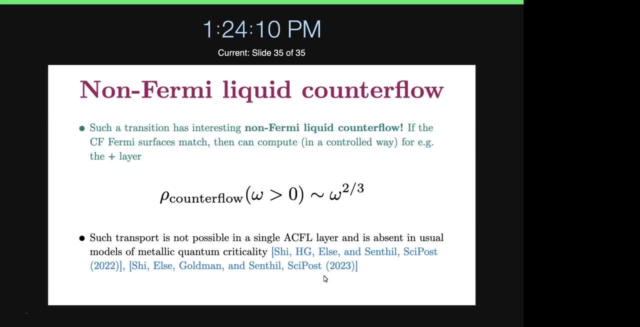 this kind of scaling in transport, which is totally universal, is not possible in the simplest models of non-Fermi liquid. but it's at quantum critical points that we study. This was shown in some earlier work, also with Darius and Dominic Els. 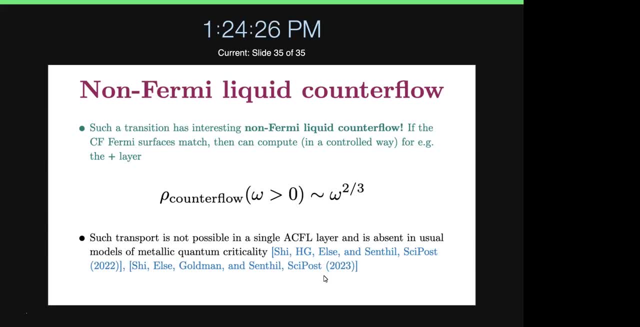 All right with that. I'll conclude and take questions. Do you know whether the composite Fermion between the high layers will be a trapping function, or will it also? Sorry, The composite- Oh, the bilayer Right, It's. also. that's why you can get this, Because in the ordinary cases you know. 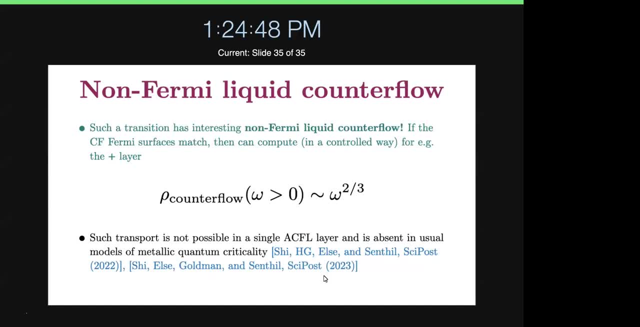 there's an exciton stability. that generically happens. That system would be-. that's why, like, if I were to take like one half on one half, this would not- because you would-. the composite Fermion is just always one pair. The point is that here, 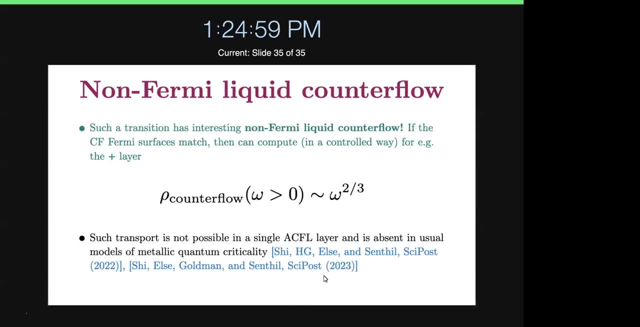 I can get a finite- a fixed point that actually has a finite exit. Yeah, that's the-. I didn't emphasize that for time, but that- that's the trick. Yeah, So do you contrast this, like fraction parallel of Romanego with the analogous fraction? 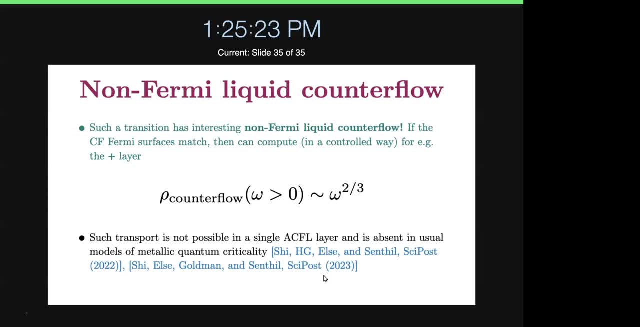 parallel, as I keep saying, or electronic systems. I think there's some subtle pieces of the bilayer and I think that sounds good, Right, right. So, first of all, this is more singular, but I think you're talking about the T to the fourth thirds. 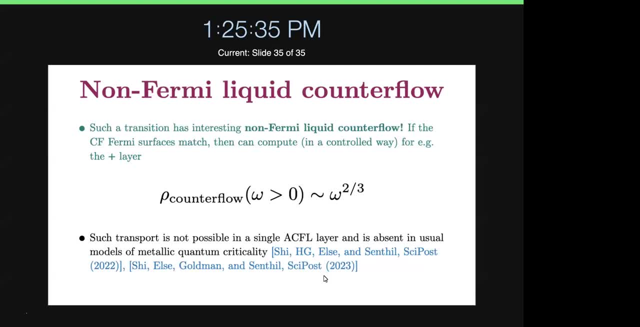 Yeah, I don't-. Yeah, I'm personally- Yeah, so you can estimate the transport scattering rate in like this millisecond period is that's like T to the fourth thirds and there's an expectation that that appears in transport, although actually-. 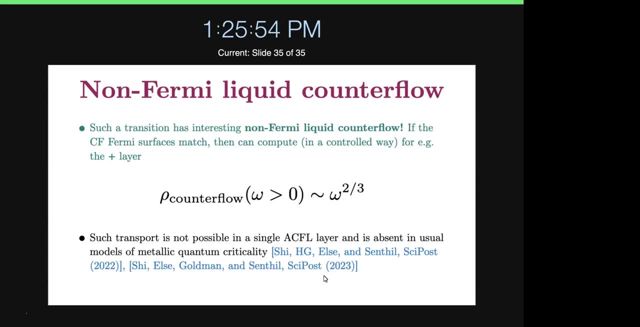 Over the years people have argued about whether it can really be there because there's no moment on relaxation. But that's not a that's not really an issue here. Yeah, it's not a Galilean invariance, so you wouldn't. you don't need for their additional. 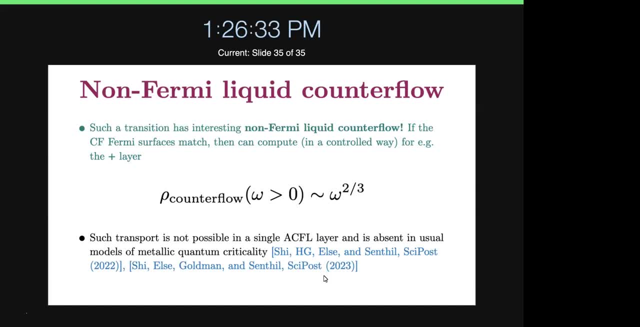 sources to get temperature-dependent scaling. I guess, even if you break Galilean invariance, if a finite momentum state carries current, then momentum relaxation is not a problem. But here you're saying a non-zero momentum state carries no current, because it's like 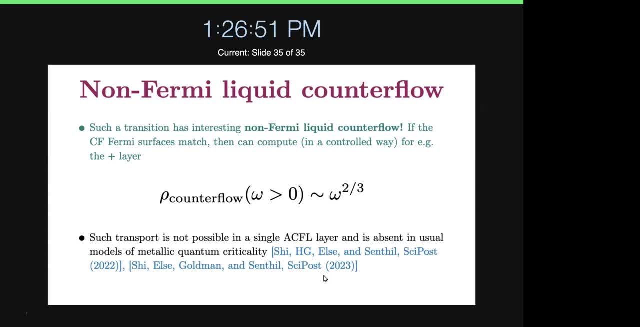 a balance between poles and what's on the scale. If we consider it to be practical in one way, we still have one function and there's a correction case where you can still have this state, I see. So the delta functions: cancel out, right. 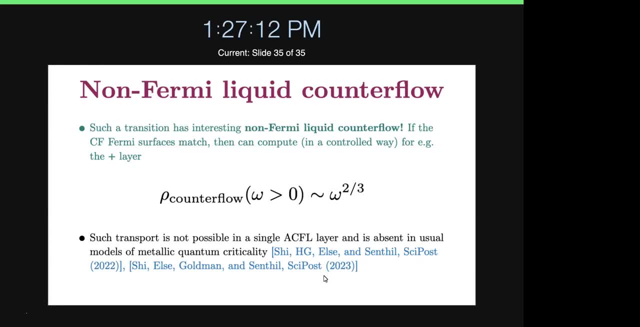 Exactly, Exactly, Yeah, Yeah, I think we have one in front of the room audience. Okay, Okay, Can I mute? Yeah, Yeah, Hi. Thanks for the nice talk, Hart. So I wanted to take you back to something that you said was already was not innocuous. 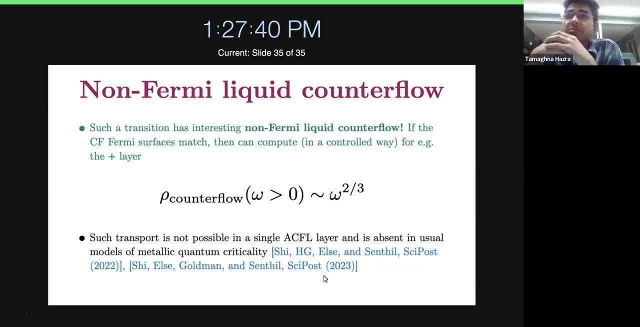 this projection into the churn band to get Cool Projected coulomb. Have you thought about how that process- I appreciate that this is the simplest thing to do and it gives good results- Have you thought about how it might be controlled? or is there some sense in other terms? 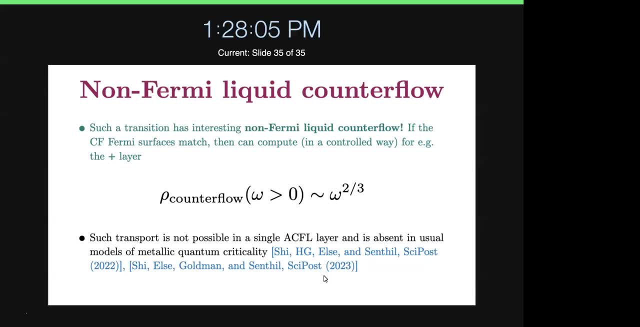 You're worried about effects from mixing on these results. Not just mixing, but other terms that might, For instance, Not be local, like correlated transport induced by a projected coulomb, things like that. Even if we don't worry about mixing, are there other terms that besides projected coulomb? 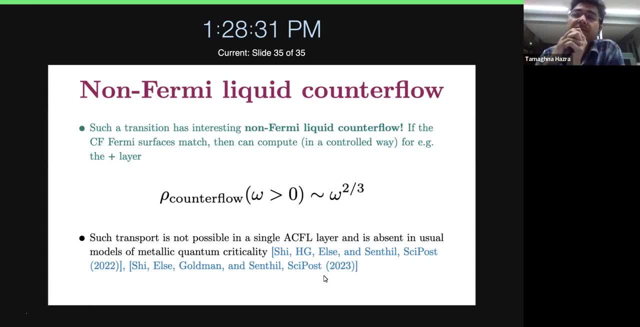 that could be relevant, could be important. So the projected coulomb is the Will always be the dominant interaction energy scale Mm-hmm. So I guess in principle you could have higher body interactions or something, but those will always be weaker than. 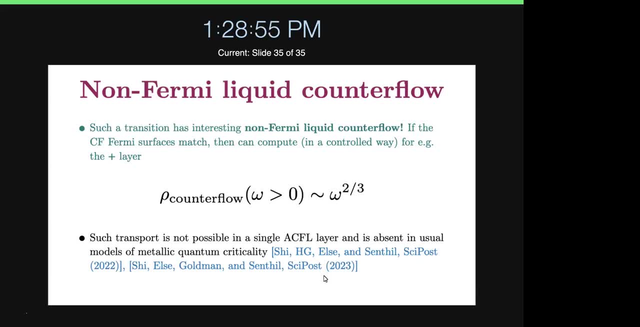 Those will always have weaker effects than the coulomb. But I mean, yeah, in principle one could try to add such things. I don't really know physically what they would correspond to, but I guess in principle you can always add anything that's consistent with symmetry there. 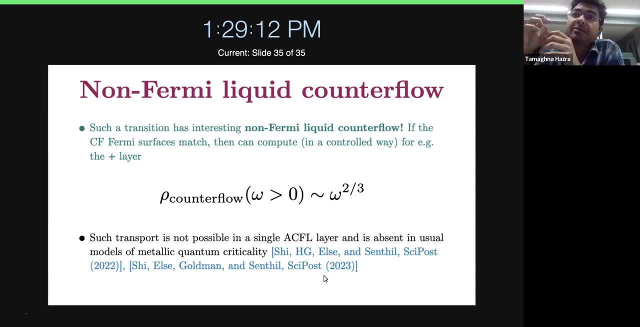 Yeah, I guess I'm thinking about correlated hoppings like density times C, dagger C or pair hoppings. Oh, I see, I see. Yeah, I have not thought about the effects of those. My collaborators may have certainly thought about this thing. 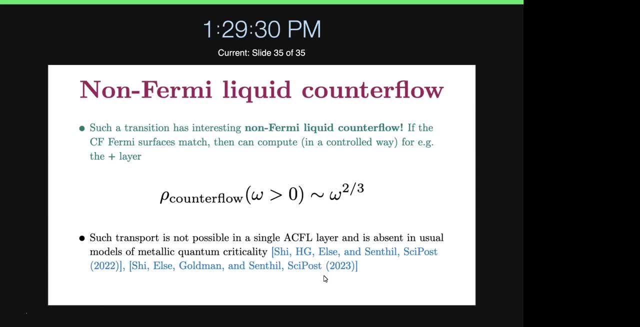 Could I comment on that actually? Oh, Nisharga, you're here. Okay, good, Yeah. So this is Aiden also joining in from Nisharga's laptop. Yeah, Hi, Hi, Yeah. So the band projected exact diagonalization calculation is done in momentum space. 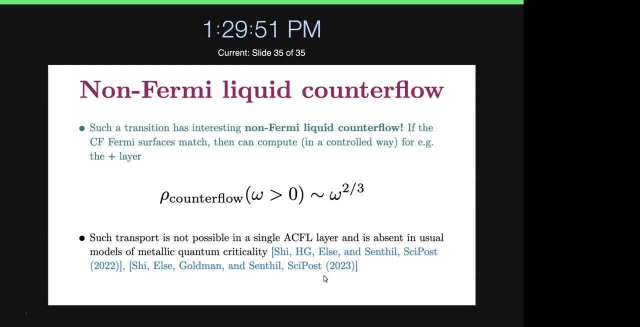 So it takes into account the exact single particle dispersion of the block states in this churn band and it takes into account all the microscopic coulomb matrix elements. It's not just putting it on a lattice and only taking nearest neighbor repulsion for. 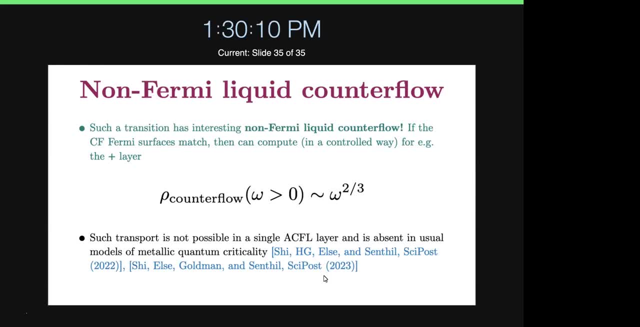 instance. So you're talking about correlated hopping terms. In principle, those are all contained in the projected interaction model. I see, I see, I see. So it's just that. have you tried turning off everything except projected density density, and does it change any of your exact diagonalization results? 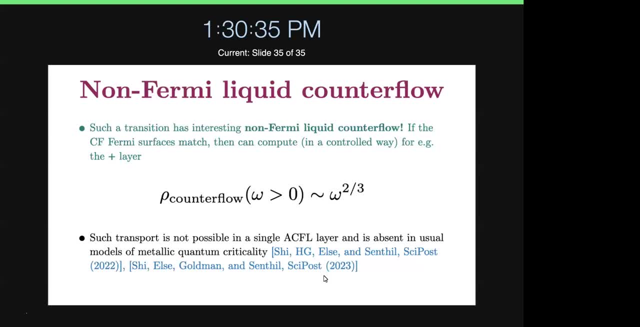 No, I haven't tried doing anything, Nothing like that, Because I think the picture that I got from the talk was that the important thing was the projected density, and that's a simple story and sounds reasonable. But what you're saying is that anything else beyond that was also included in the ED. 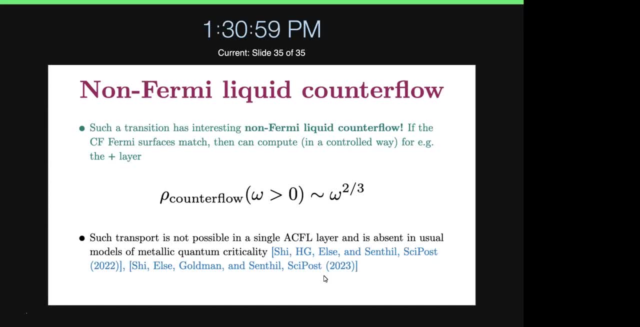 And I just didn't catch that. Yeah, The interaction that we're projecting is a standard coulomb interaction, And once you project a coulomb interaction into a band and the wave functions of that band aren't just delta functions at lattice sites, then you always end up with these interaction. 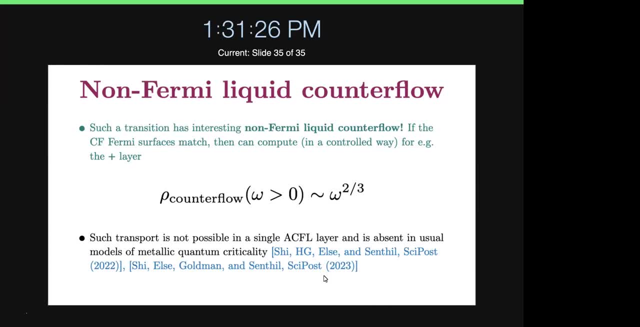 terms that don't really look like density- density interactions if you were to write them in a lattice model, But they always originate from just a standard density- density- coulomb interaction when you have wave functions that are not perfectly localized. Got it, Thanks? 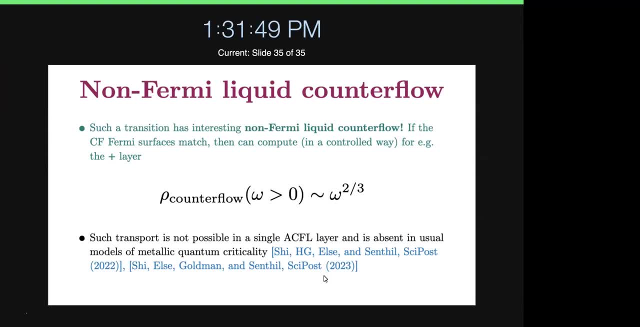 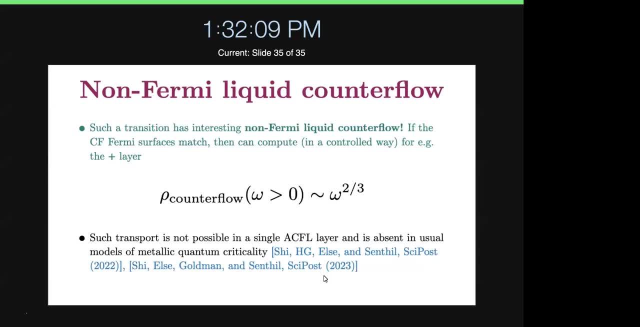 Aren't you my collaborator? Why are you asking me questions? Yeah, Face♥. I just on the merits. Okay, Not something I did. So there was one Face força. I can do the two thirds. you see, a regional compensator. 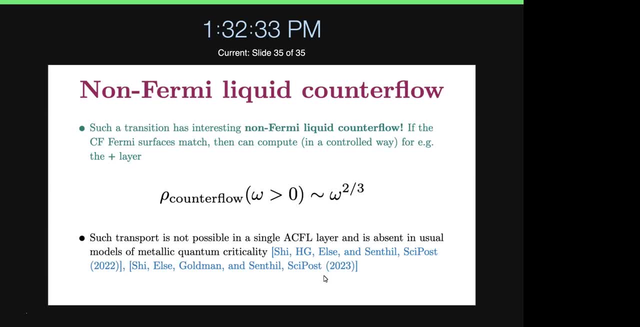 Is there a qualitative understanding of what's going on? There's a strong particle symmetry branching- Actually Aiden wrote a separate paper on that- but you can see it fairly naturally just analytically. So in the experiments they also try to. 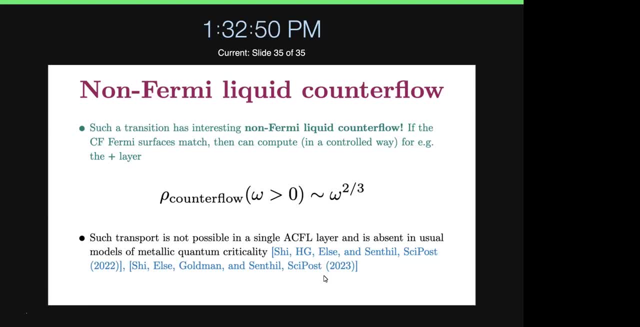 so they solve two-thirds. Do they try to look for one-third? Yeah, I mean, presumably if you go by in Numerics you go to more optimal twist angles. But is there some approximate particle symmetry that's optimal twist angles? I believe particle symmetry is still broken. 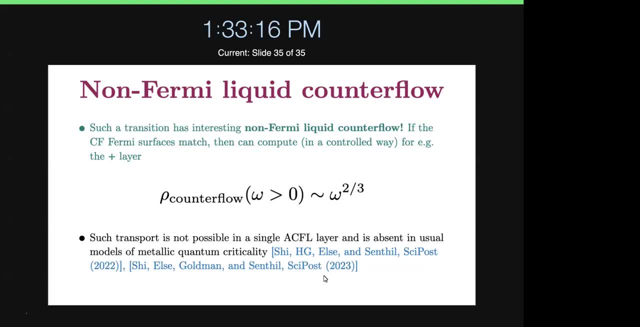 Aiden, is there a sense in which you think that there's an emergent particle symmetry or something at two degrees, or Yeah? so two things that I'd like to say. First is there is some experimental evidence for a charge density wave at filling factor one-third. in devices where there is a fractional quantum anomalous Hall state at two-thirds. So in particular you can take a look at there's a Nature paper from the group of Kin Phi Mac and G Shawn And yeah, so there is some evidence. 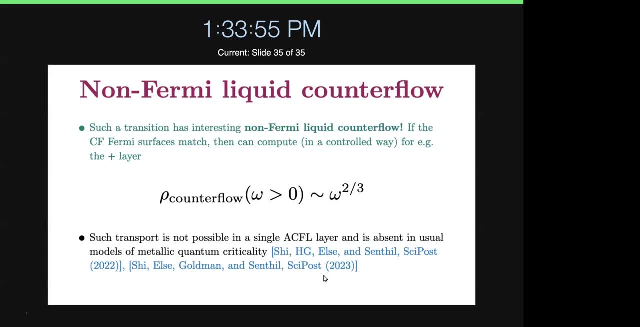 for that charge, density wave state. experimentally, Regarding the question of some sort of particle hole symmetry, what we find is that near some magic angle, if you'd like to call it that, which, given the DFT parameters that we're using, seems to be somewhere around two degrees. 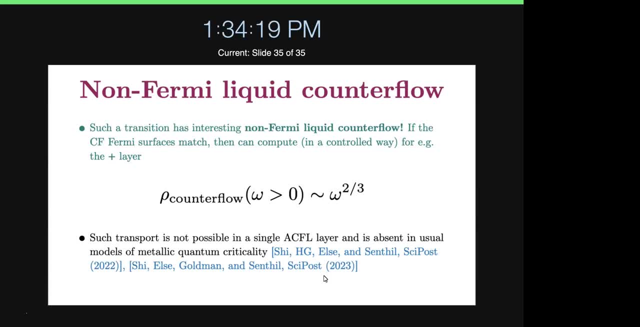 but there's kind of a big error bar and uncertainty on that, I'd say due to just uncertainty of the DFT parameters. But if you take our model and you go around this magic angle, what you find is that and you do band projected ED. 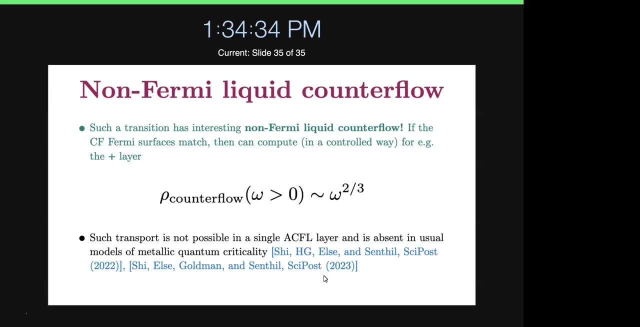 what you find is that at every filling fraction, the system seems to be almost identical to band projected ED of the lowest Landau level, And because the lowest Landau level, and any Landau level for that matter, has particle hole symmetry. when you're close to this magic angle, 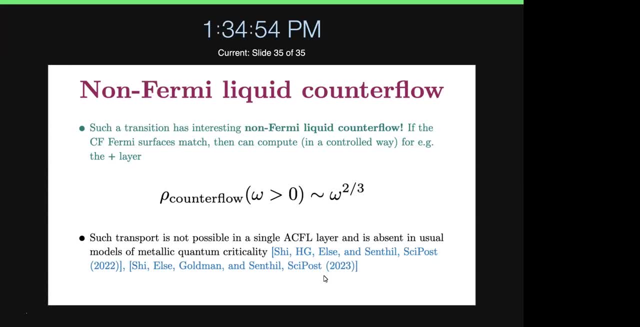 the TMD continuum model also seems to have approximate particle hole symmetry, and that's what we're looking for. And that's what we're looking for is a particle hole symmetry. Well, I guess that's the question: whether there's ever a sense in which it's exact. 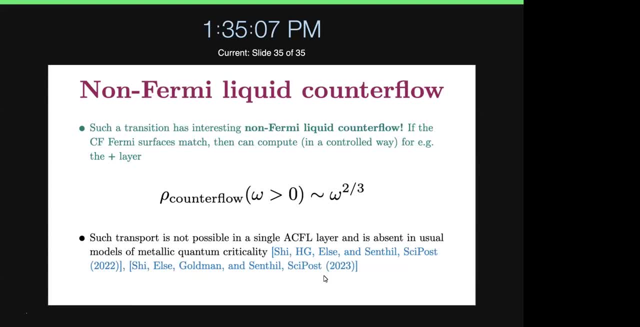 I don't think there is. Yeah, I don't think it's ever exact, But basically what I'd say is, when you get close to this magic angle, the band projected model becomes almost identical to the band projected model of the lowest Landau level.